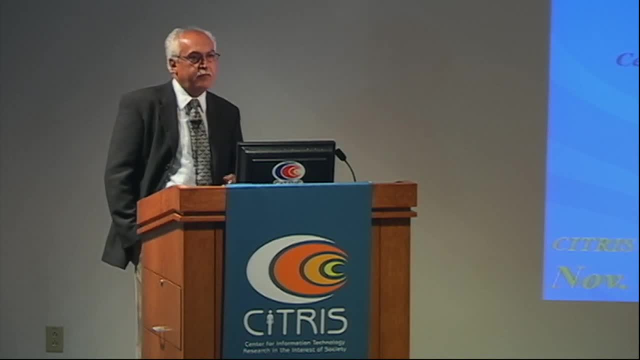 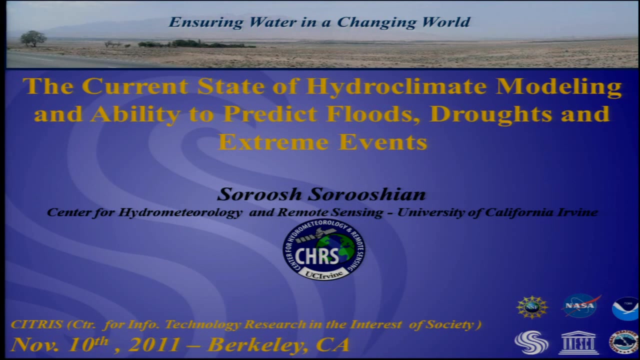 was there. My original work was on rainfall runoff models, particularly for the National Weather Service. I also worked on the water resource hydrology for flood forecasting. Anyhow, the topic that I chose today is really the current state of hydroclimate modeling and our ability to predict floods and droughts. Those are key hydrologic issues that fall. 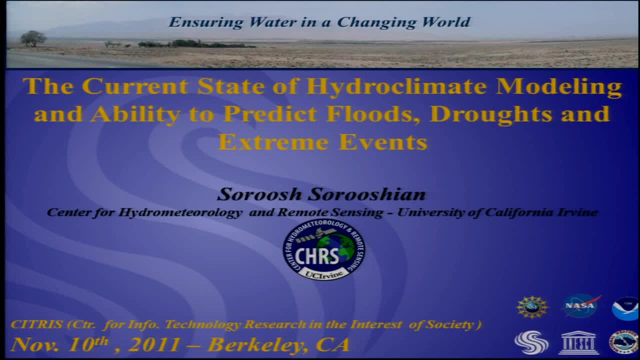 in the context of, perhaps, the extreme events, and I'm humbled to be in a place where there's so much work going on, particularly on climate modeling. But these, to some extent, are not the best models And to some extent may reflect my own, some of my own personal views as well. Funding: 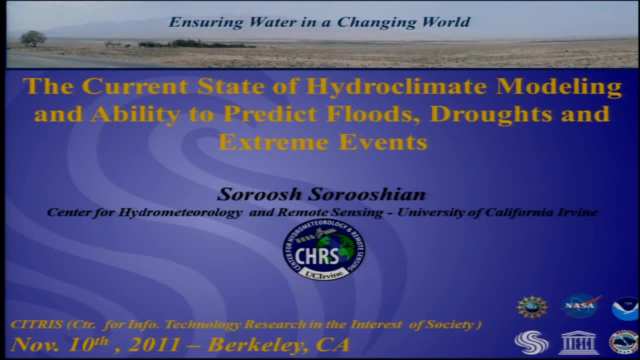 for some of my work comes from NSF, NASA, NOAA, And we have collaborations with UNESCO. with respect to the work we do for the center, And while I'm not talking about some of the research in my group, but it's been primarily focused on retrieving precipitation or rainfall- 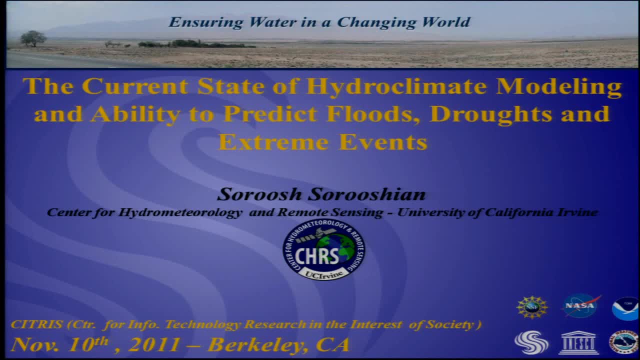 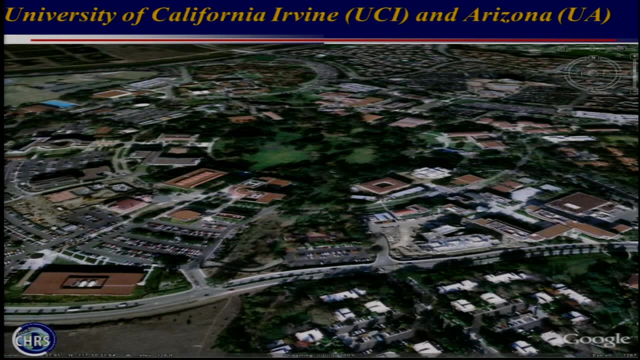 estimates globally from satellites. Thank you, And if you type in CHRS, UCI, I'm sure you'll go to that website. I come from UC Irvine, as you know, and previously was at the University of Arizona for 20 years. 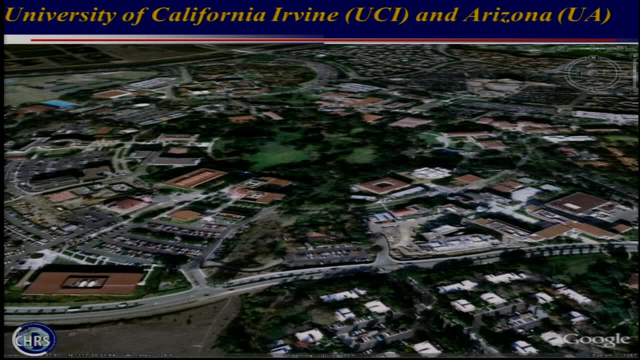 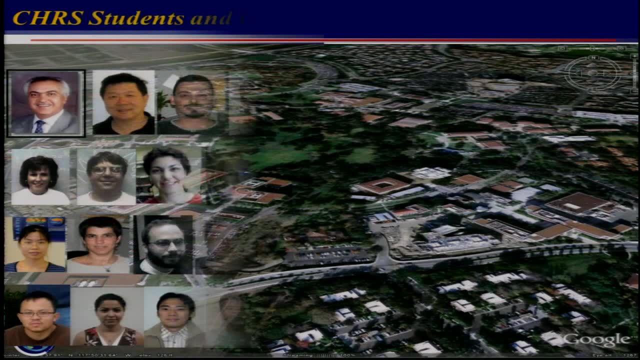 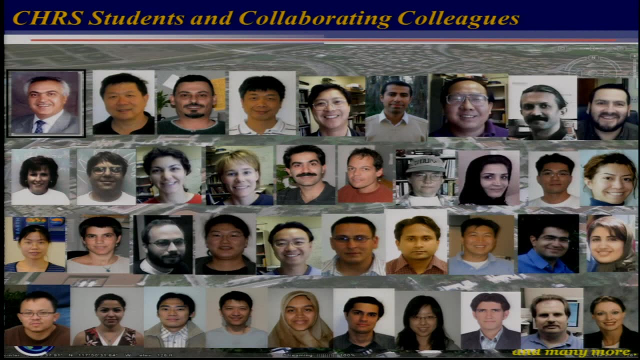 And that's where I had the pleasure of working with Roger Bales, who is in the audience, And we both departed Arizona about the same time And I usually like to acknowledge some of the students and collaborators with me, And so some of the slides they prepare for me I better acknowledge what they do for me. 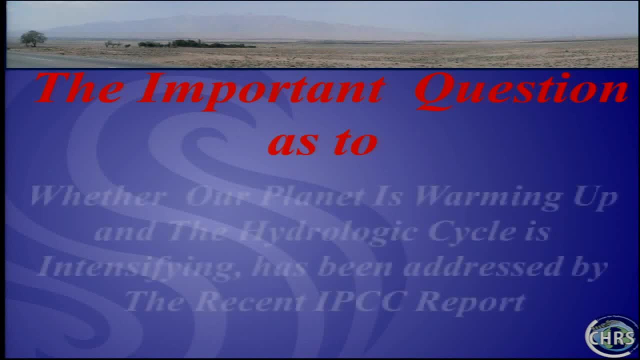 The important question as to whether our planet is warming up and the hydrologic cycle is intensifying has been addressed by the most recent IPCC, as well as by the US Department of Health And many others, even though, unfortunately, due to some circumstances. 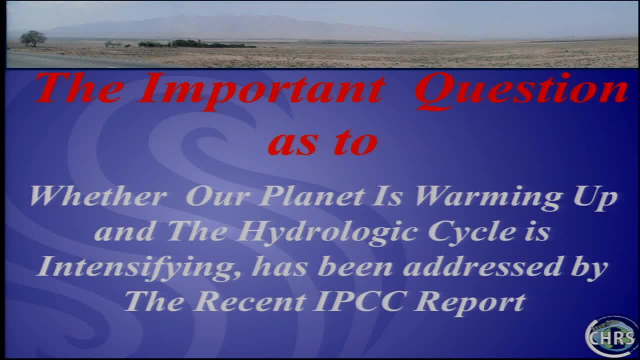 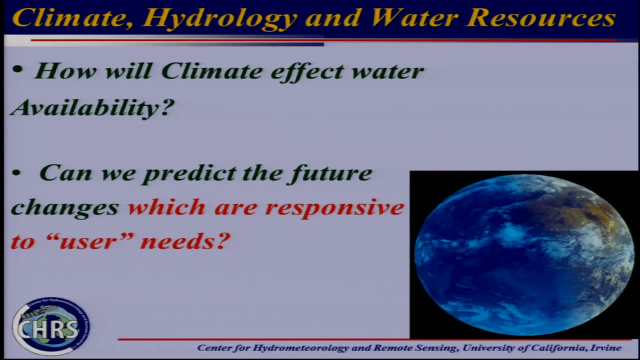 some doubt has been created in the minds of the public, But the realities are that warming has happened and there are, as you will see from this talk, maybe there are- some evidence that perhaps the intensification of the hydrologic cycle is something that is likely happening. 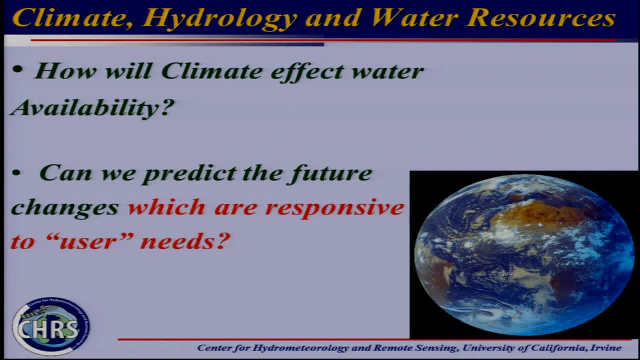 Okay, So how do these things affect the climate, affects water availability, and how do these things affect the environment? And can we predict the future changes which are responsible to user needs? Because, after all, no matter what research we do, particularly in the area of water resources, 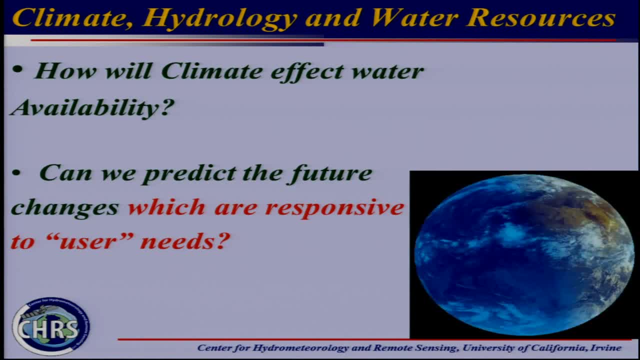 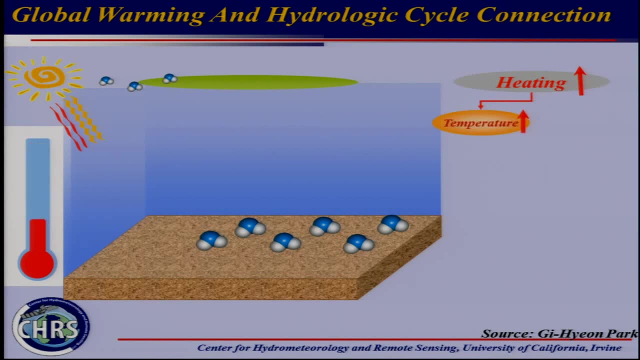 and its connection to climate change has a human aspect to it, and society certainly would like to know how to address these things In terms of the connection between hydrologic cycle and the climate, global warming. it's pretty straightforward physics, Of course. if the temperature goes up, obviously the amount of evaporation 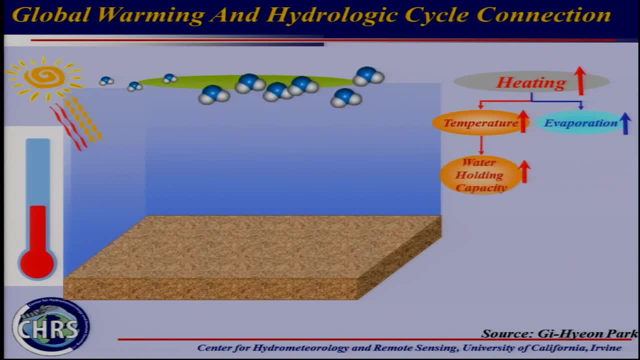 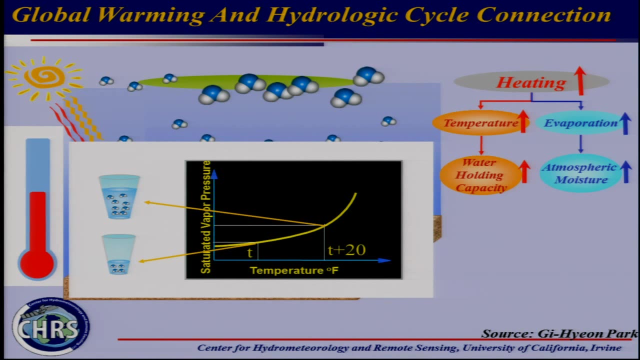 given we have quite a part of our planet covered with water. it's simple physics that it happens. And also, as the warming happens, the water holding capacity of the atmosphere increases. Roughly. for every 20 degrees increase Fahrenheit in temperature, you double the capacity of the atmosphere. 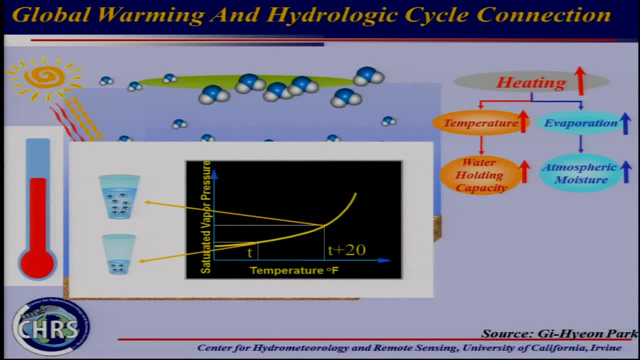 So with the two of them combined, the more you have there obviously under residence time, water in the atmosphere being 20 days. what goes up must come down. So the expectations are that, as a result of the global warming, you expect that the global amount of precipitation to increase. 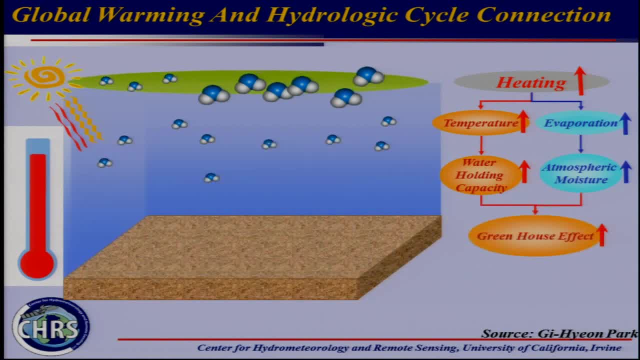 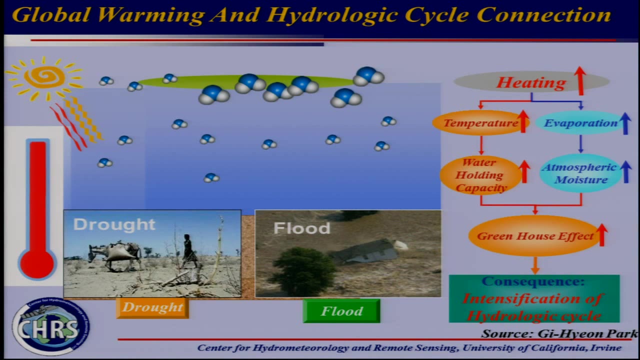 Where it falls is the million-dollar question of the concern, And water also is a greenhouse gas itself, and so you can imagine with the other gases, what role it plays is going to be important. So, from people who have been working on this problem, 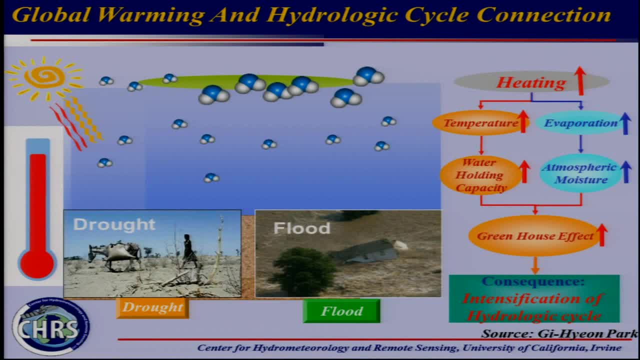 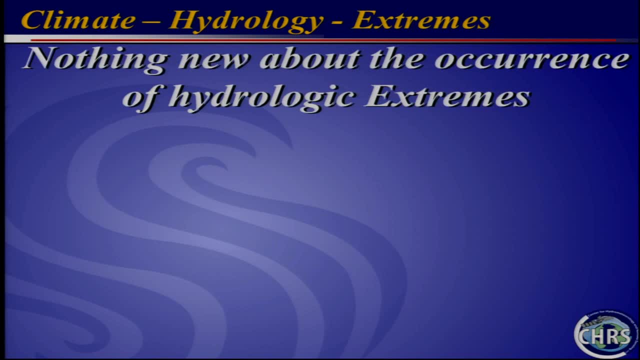 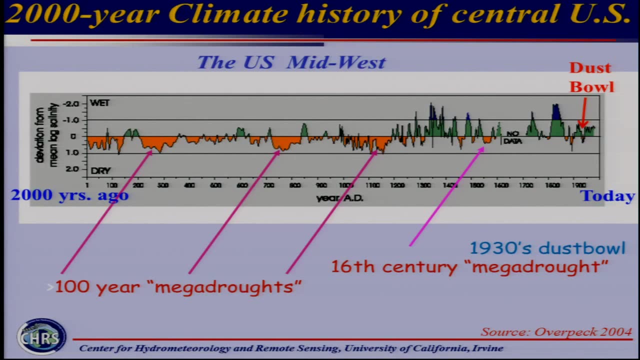 they say. well, as a result of all this, it is likely that we're going to be seeing the intensification of the hydrologic cycle, which is really nothing new about the occurrence of hydrologic extremes, and that's really what the focus of much of the interest is. 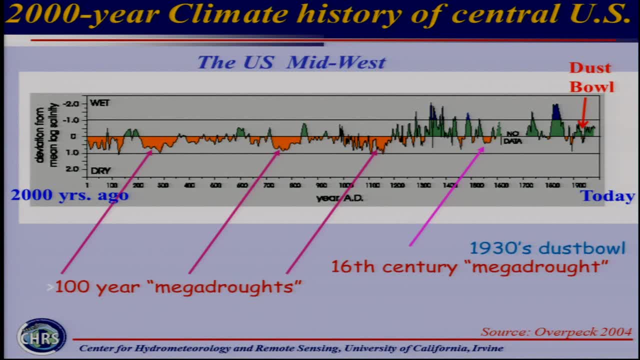 When I say there's nothing about hydrologic extremes. if you look at this 2,000-year reconstruction from actually some lakes in the Midwest US- and that's attributed to my colleague in Arizona- Over Peck, they have reconstructed based on the Palmer Index. 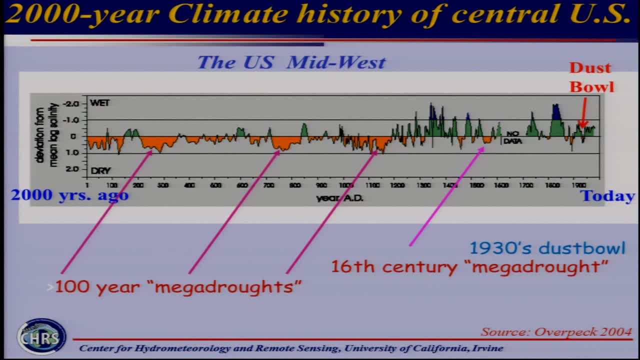 where anything that's below the line is the areas of dryness, and anything above that, with respect to this particular scale, is times of the interweaving. So you see that in the past, based on the isotope work that has been done, 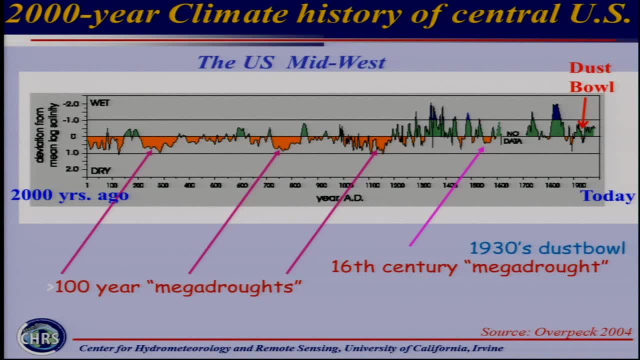 there are lots of periods of time where sustained drought that has lasted hundreds of years has existed and if you look at our most current time, Dust Bowl really is pretty tiny with respect to some of the things that have been experienced in the past. So extremes in even the 2,000-year span of time in North America or US are not really unusual. And of course, in the past 100 years or so we have been enjoying a more wetter period, and perhaps this is of some concern. 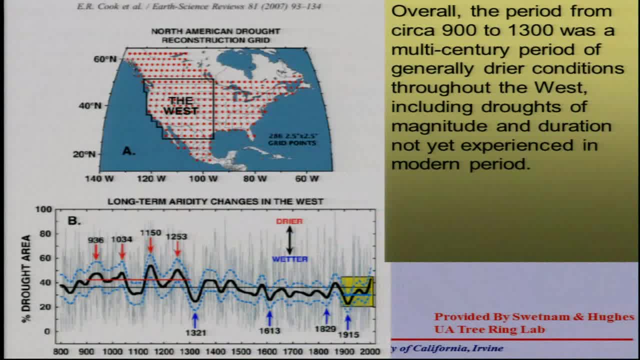 And the tree ring work that people again at the Tree Ring Laboratory in Arizona have done. looking at this chunk of the western United States and the way this graph works, it represents the percentage of the area that has suffered from the drought. 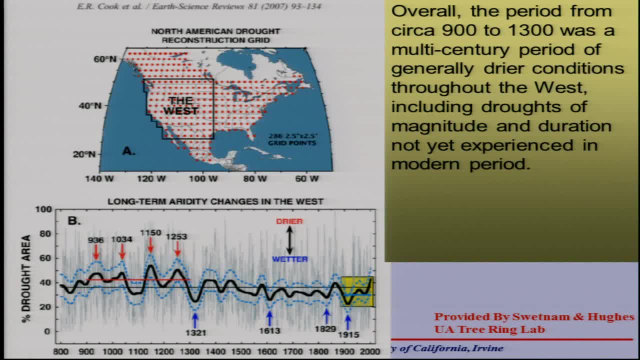 So if you look, these are the higher percentages. So there have been periods. they're ranging from 900 to 1,300-year multi-century periods, generally drier than average, and those are consistent with what has happened in the central part of the US. 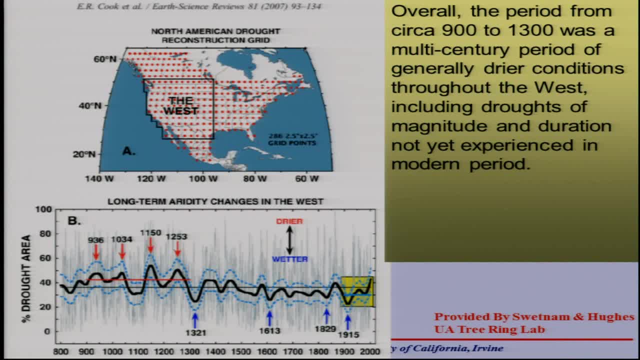 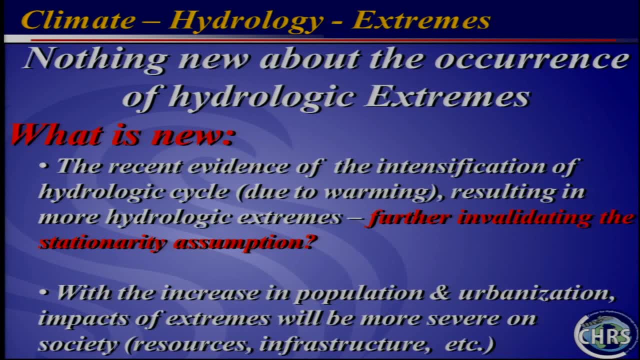 So extremes are there and maybe we've been lucky in the past 100 years that we haven't had as severe of these extremes. That happens, Okay. so what is new about all this is that the recent evidence of the intensification of the hydrologic cycle 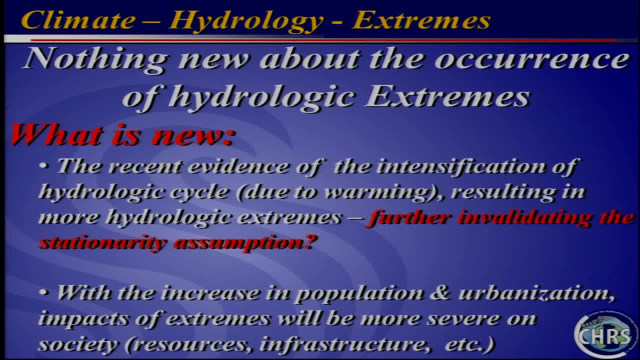 is more about the extremes And it's further invalidating the stationarity assumption that you really cannot assume all the time that nature behaves in a stationary fashion, because a lot of our methods and methodologies and models are based on that. But the question is what alternatives we have. 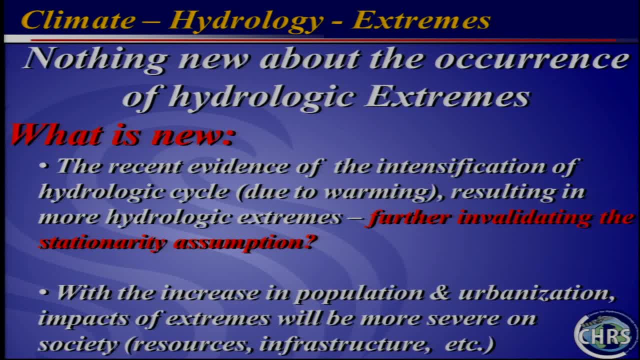 how much time we're putting into trying to resolve design criteria et cetera. I'll talk about that a little bit later. And then, with the increase in population and urbanization, impacts of extremes will be more severe. Obviously, the more you pave, the more roofs you put. 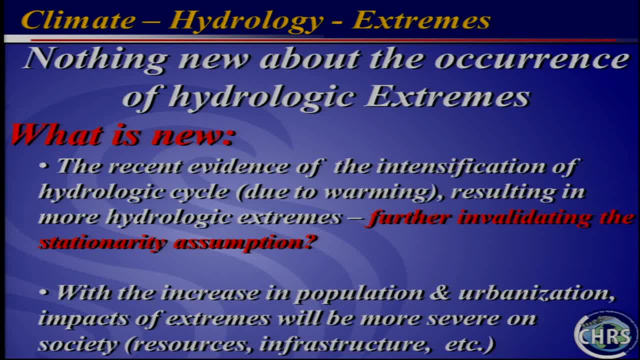 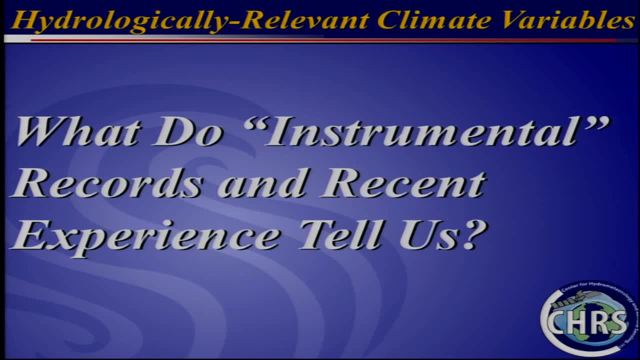 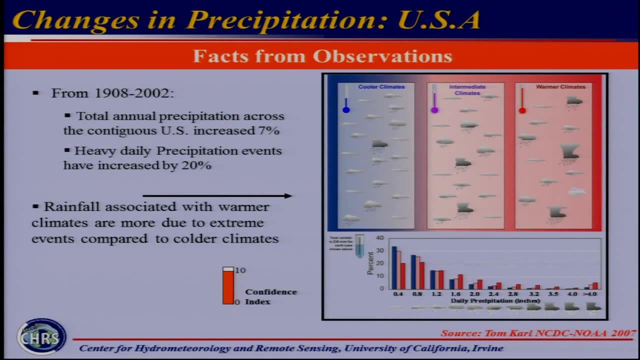 you're going to also add into the non-stationarity aspects and it becomes an issue with respect to infrastructures and others. So, looking at the history- at least instrumental records- what does experience tell us? And I borrowed this from Tom Call: 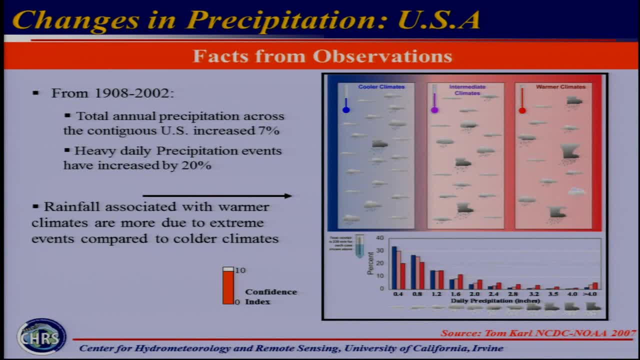 who's the director of the National Climatic Data Center And their analysis. they pretty much have all the rainfall data over the United States and globally. they collect the data And going from 1908 to 2002, and I haven't been able to get an updated version of it. 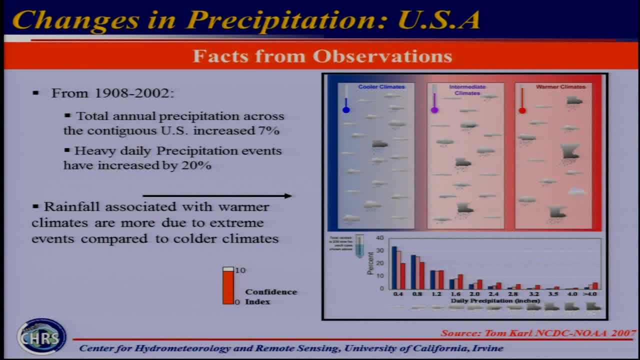 if you look at their historical gauge data, it shows that the total annual precipitation across the United States has increased by 7%. So to some extent it validates this business that with the warming that has taken place it happens that also with the US. 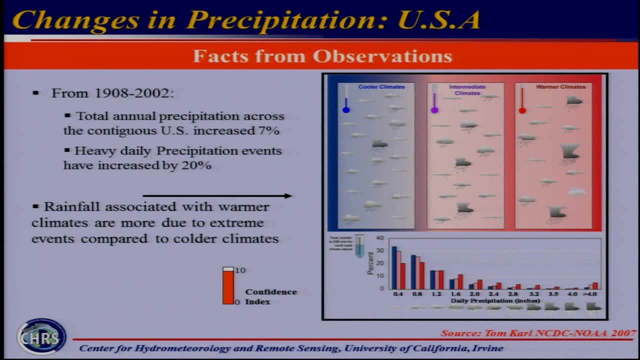 we have benefited from more precipitation, But more importantly is that the heavy daily precipitation, you know, the more extreme cases have increased by 20%. Okay, And this is the issue of the intensification that we were talking about. And again, 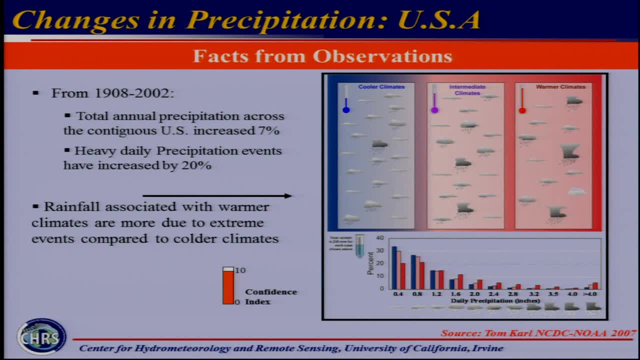 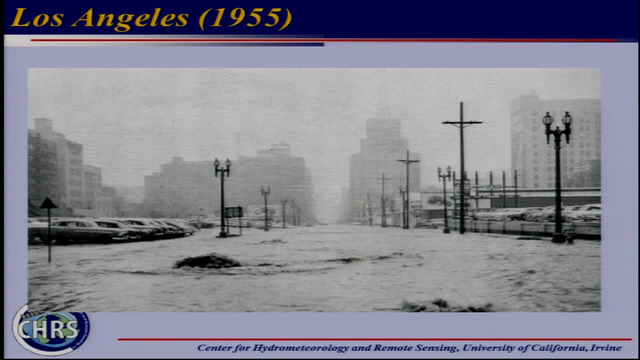 the rainfall associated with warmer climates are more due to extreme events as compared to the colder regions. if you wish, And you know, extremes have happened. 1955, downtown Los Angeles. I guess I wasn't in the US at that time. 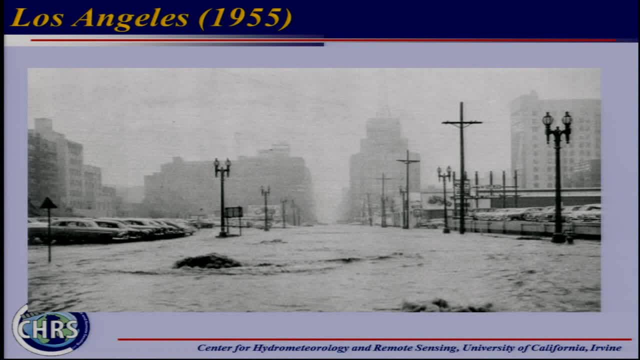 And I assume people who have been there must have experienced it. We've seen extremes in Manila, I mean in Philippines, this past few months or so. it's been really extreme. And then if you look at, say, 2007,. 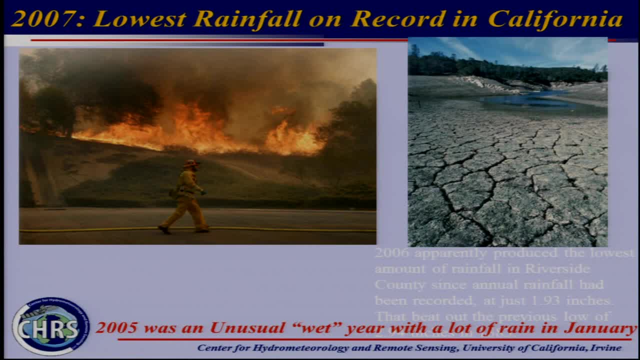 we've had the lowest amount of rainfall on record in California, And then 2005,. two years earlier was perhaps one of the wettest Januaries we had. We got the amount of rain in a matter of three days that we would have had in a matter of the whole season. 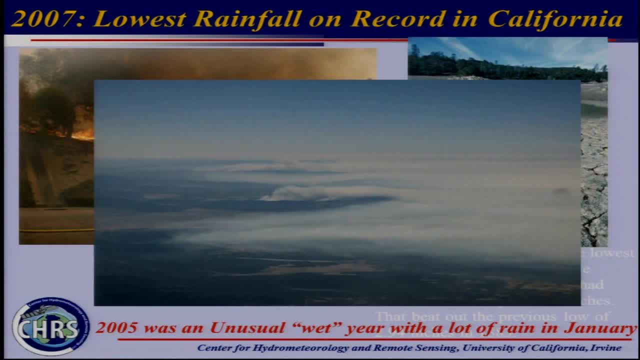 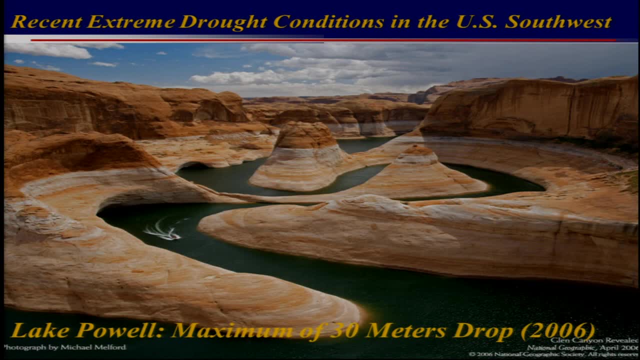 So we had a lot of fires and, of course, made quite a bit of national news, And then the main source of water for the Western United States being the Colorado River, it's the Lake Powell, And you know, in 2006,. 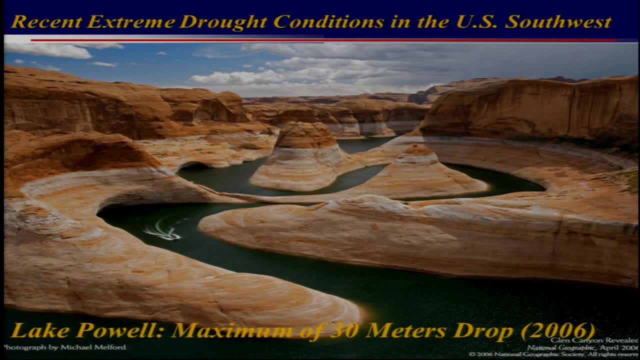 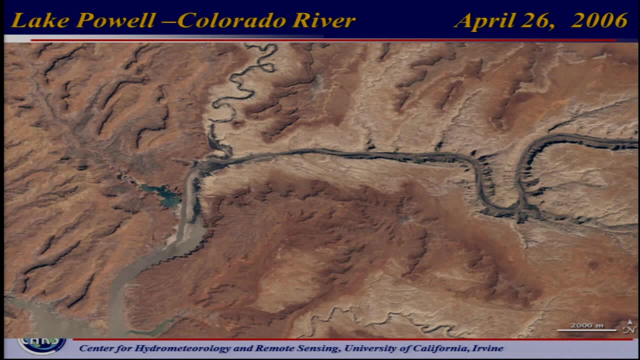 the lake level had dropped by 30 meters, which is quite a substantial amount. What I have next are a series of satellite views that are from 2006,, which was corresponding to the worst year. You see, the lake used to cover all these areas. 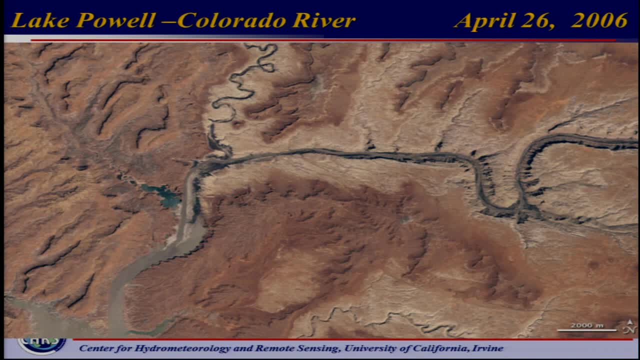 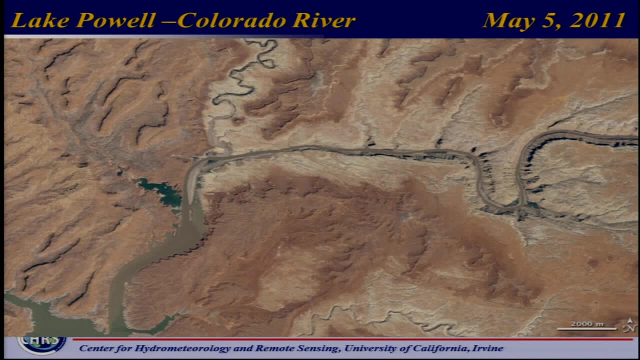 and now it's receded so far back that you know we don't have any If I go to, let's say, May of 2011,. just recently, we see at least there has been some recovery, And if you go to the good days, 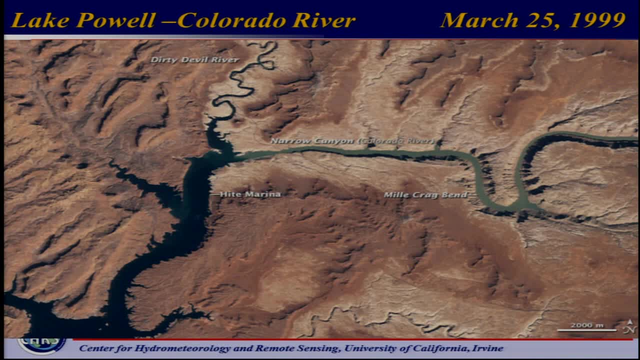 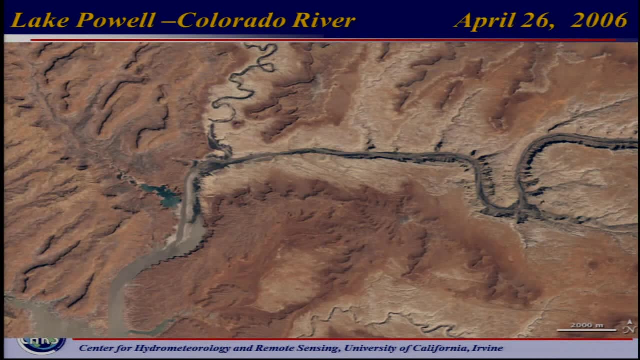 which is 1999 as a reference, you see that the lake actually went back that far within the canyons, And so just quickly again, this was the worst year and of course we are recovering, but we're still way, way below. 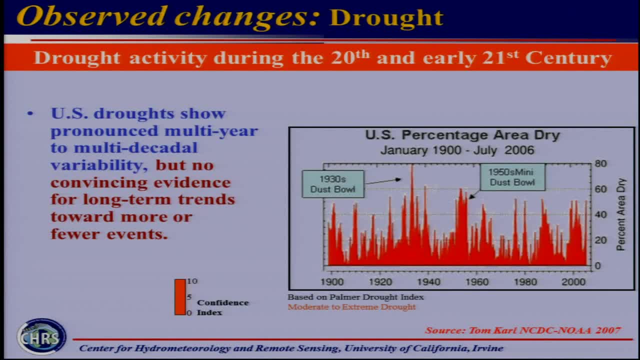 And what I show next is that, looking at all these together, the same group at NCDC have also analyzed the records with respect to the droughts, And the problem with the droughts, unlike rainfall, is that it's not that easy. 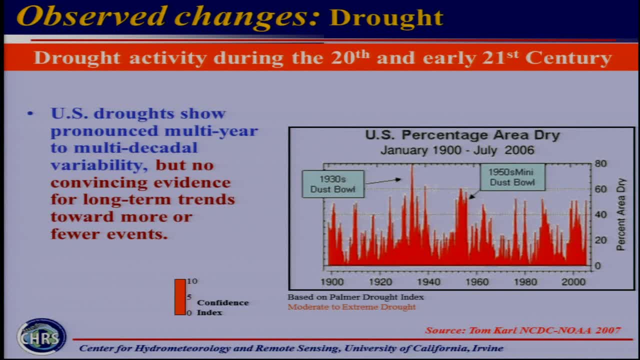 Droughts you have to have multiple number of years before you realize it. But based on the analysis again Tom Carr's group has done, they've seen from the data that the droughts show pronounced multi-year to multi-decadal variability. 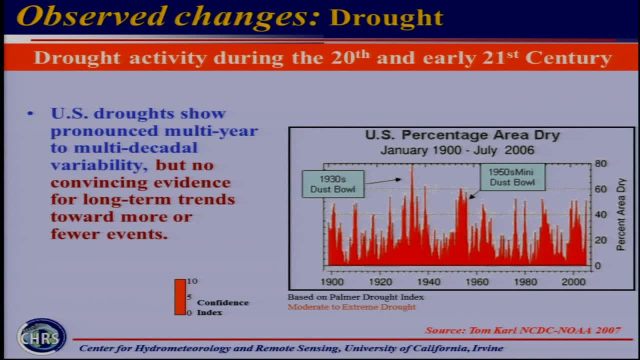 But there is no convincing evidence, based on the analysis they've done, that there is a long-term trend towards more or fewer events. So they come and go, but luckily we don't see those that I showed you in the 2,000-year historical construct. 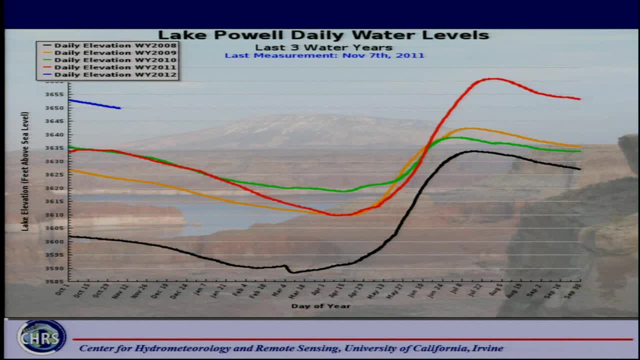 If you wonder what's the current state of these major reservoirs on the Colorado River, these colors, if this is the worst year, of course, of the height of the reservoir, the lake level, And this year has been perhaps one of the better ones, 2011,. 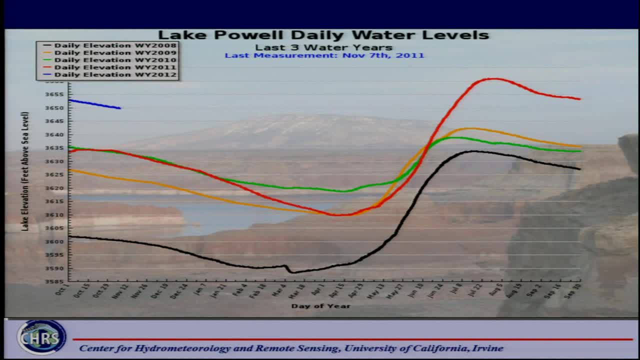 where we have recovered quite a bit, but certainly not close to where it should be. It's still 50, 60 feet below where it should be, And this is the water year always starts in October 1st and that's exactly the way it's going. 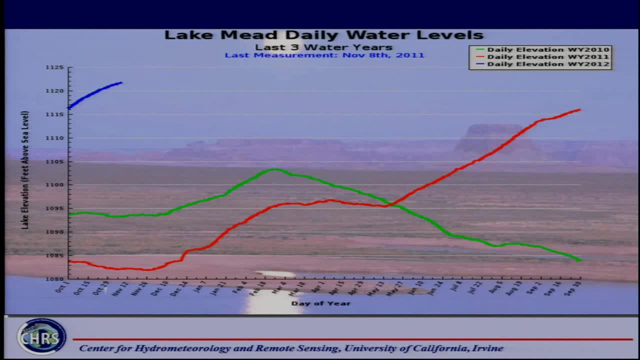 And part of the reason you see a decline there is because they're releasing more water And you know Lake Mead is actually picking up that water because of the treaties they have with the lower states that they have to get some of that water. 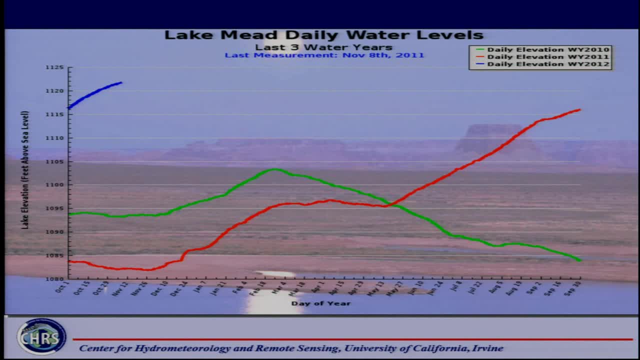 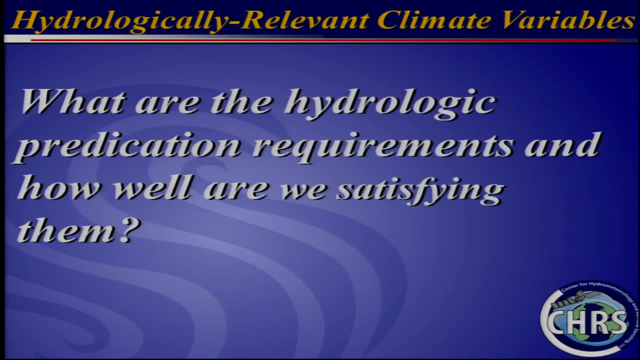 So hopefully this year this will continue on and we will have a little bit more recovery of that. So at this point I'd like to shift gears. I mean, this is what history tells us, based on 100 years of instrumental records, and for hydrologist precipitation. 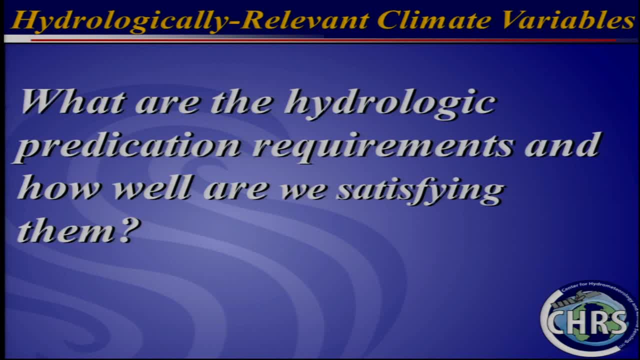 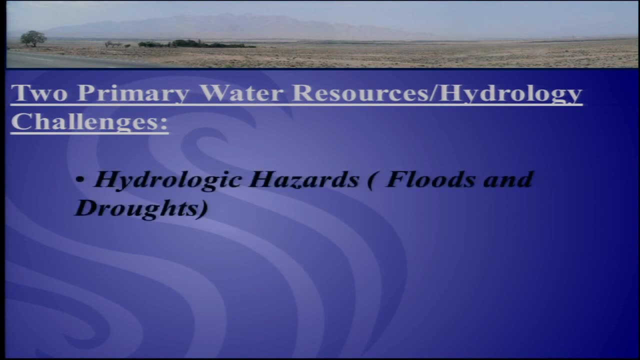 And precipitation is the most important thing. But let me go and now talk about what are the hydrologic prediction requirements and how well are we satisfying them? There are two primary water resources hydrology challenges we face. The first one is hydrologic hazards. 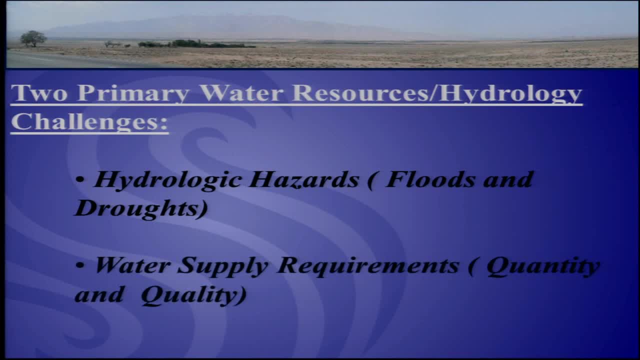 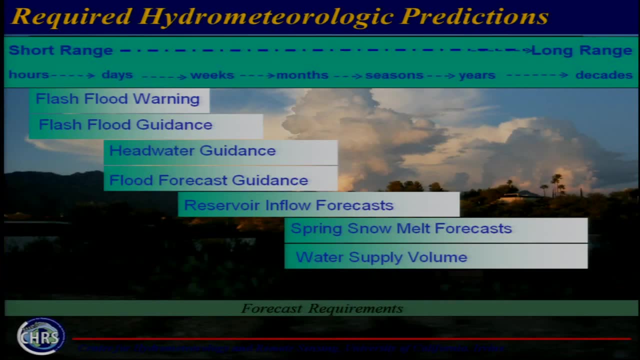 We talked already about floods and droughts, So you need to have the tools by which you can actually make predictions Ahead of time. it always helps to plan, And the second part is, of course, the water supply requirements. Let me go and present it in terms of time scales. 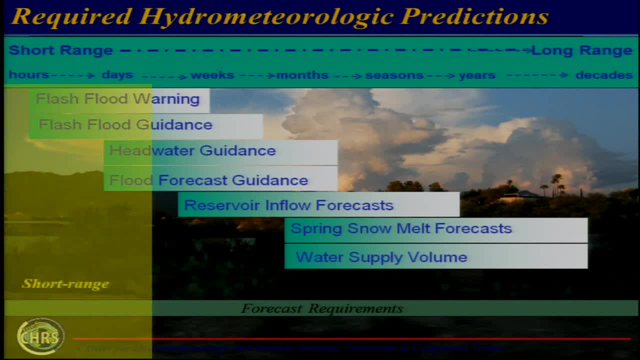 I break this up into really three zones: Essentially the short-range forecast requirements that really fall in the range of days for flood forecasting, flash flood forecasting and very much interest to the National Weather Service and for river forecasting. The second, I call it pretty much the mid-range. 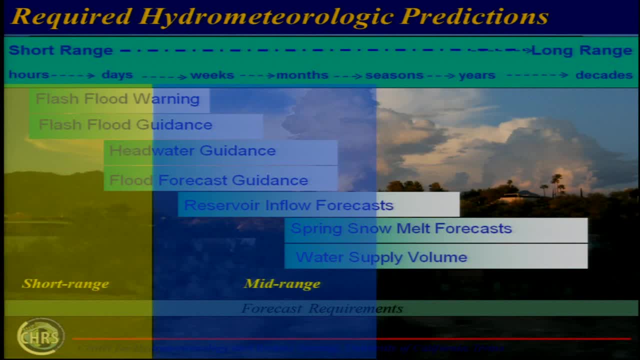 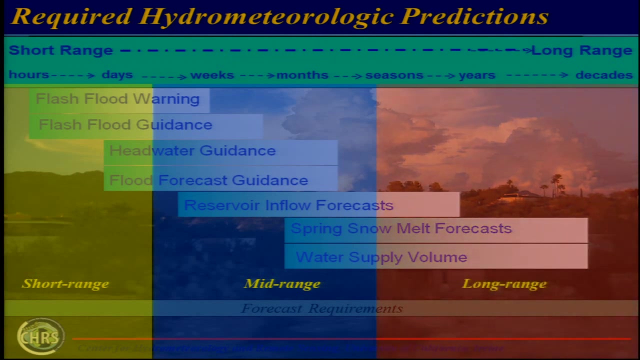 which are from weeks to months, you know, maybe two or three months, And these are known as the seasonal forecasts and important for more shorter-term reservoir operations, agricultural irrigation- And then you get into the last part, which I call it the long-range forecasting. 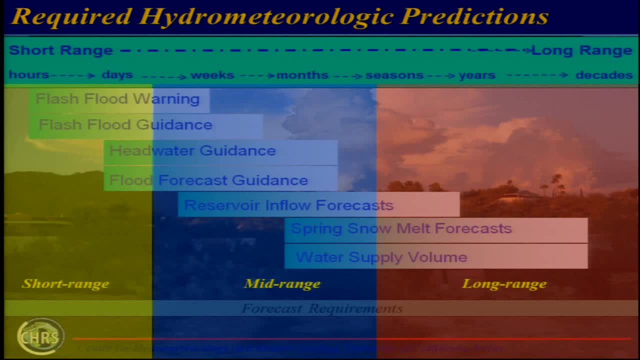 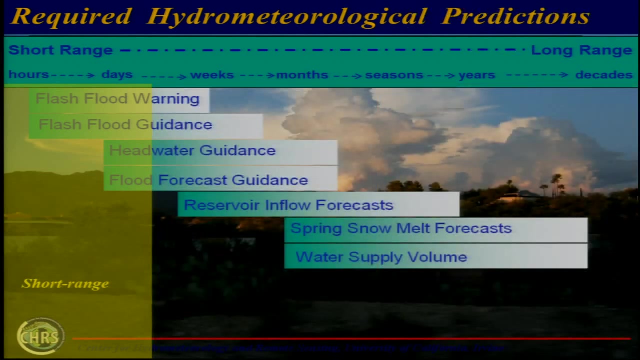 which are years to decades and centuries, And that becomes very important with respect to the planning and infrastructure design. So for each of these ranges, you have different types of models and different groups of people working on different things. Let me start with short-range forecasting. 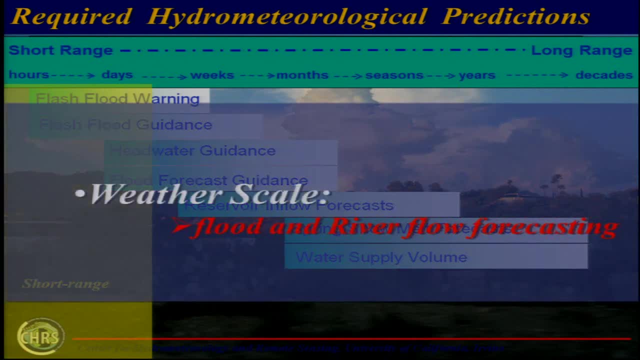 And it's really at the weather scale And that's floods and river flow forecasting, And I have, of course, a biased interest in this because that's where I started much of my work and still some of my students are working on these topics. 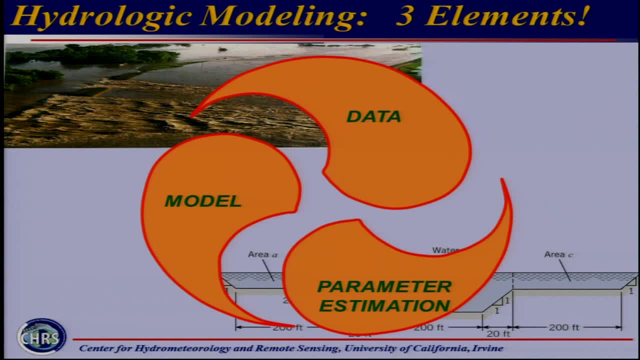 And we collaborate with the US National Weather Service. So essentially, there are three parts to a hydrologic model that is used for those kinds of forecasting. There is, of course, from a wide range of models that are available. you have to select a model. 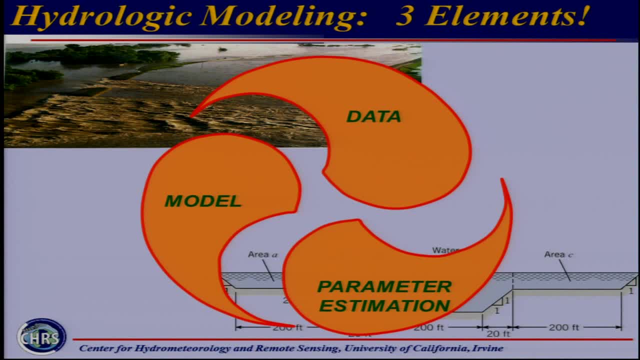 You better have the right data for the model, okay, as inputs, and also data to calibrate these models, And calibration, which I call it parameter estimation, is a crucial part of it. okay, So, if you have these three elements, hopefully, hopefully you will be in a situation. 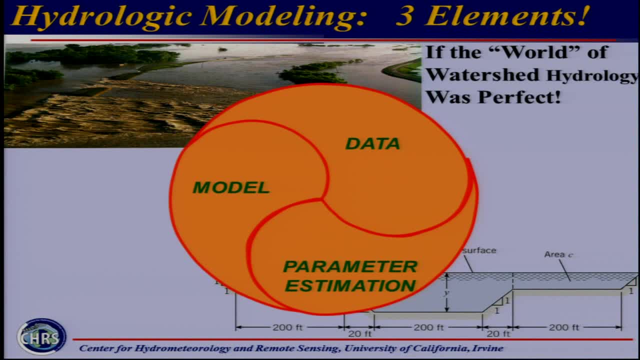 that if you can fit all three of them together, you will have the perfect model, which, of course, is never the case, And I try to show that through the two pictures. That's natural river and that may be the way we model it. 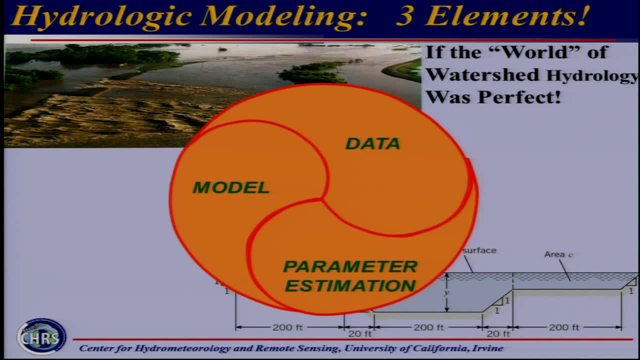 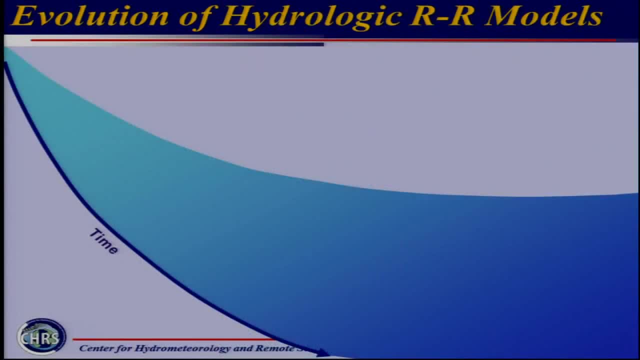 and they have nothing to do necessarily with each other. So, but at least that's the direction we always try to push- try to come up with models. So over the years, hydrologic models have evolved, starting from very simple engineering-based tools. 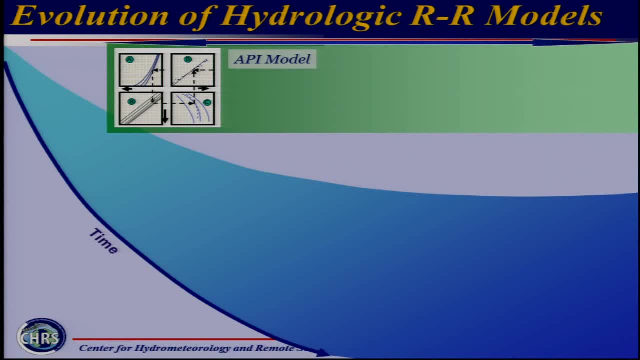 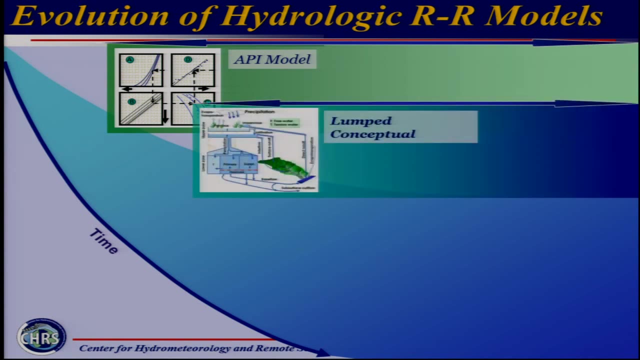 such as the Antecedent precipitation index model. That is pretty much a graphical approach of trying to get some estimates of what the runoff capacity from a water bay shed would be. And then, with the advent of digital computers and the work at Stanford with Linsley, 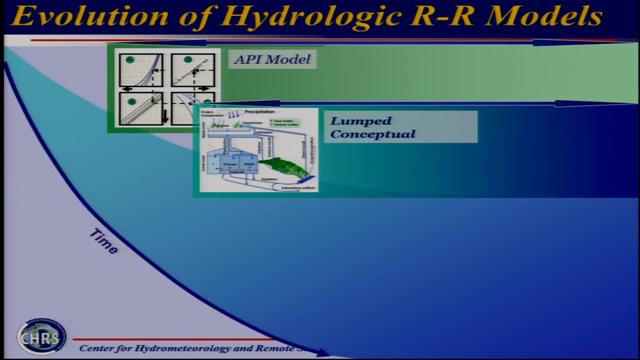 Ray Linsley and Crawford came the first generation of conceptual rainfall runoff models that are lumped in nature. They assume everything is averaged over the basin and fed into a model, because then you can have parameters all the same. And then, more recently, with more advanced computers, 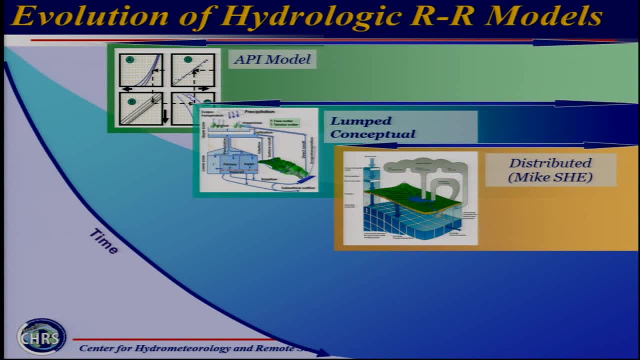 better observations. people have started. well, nature doesn't work that way. You know. we have heterogeneities on the basin or on a watershed, and therefore we better reflect that Rain never falls uniformly over an area, so you better take care of that. 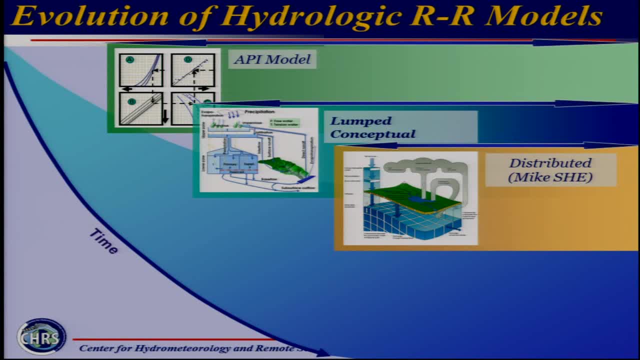 So we come with a whole host of distributed hydrologic models And with requirements like Norm Miller and others have with respect to climate modeling, then you have to have models that give you a better interface of the land surface hydrology with climate models. okay, 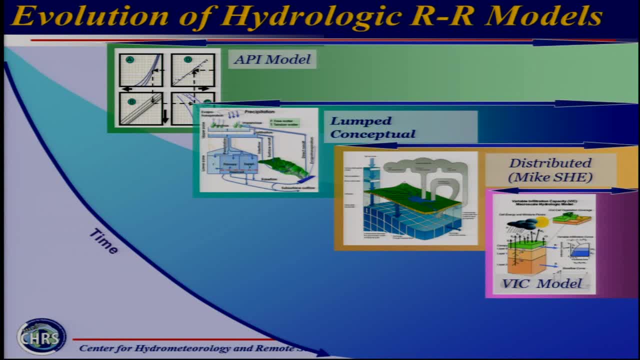 And these are the type of models that have been developed to take care of that aspect. So over the time we've gone from really lumped type of models, mathematically speaking, towards distributed models, and we've gone from simpler models to more physically based models. 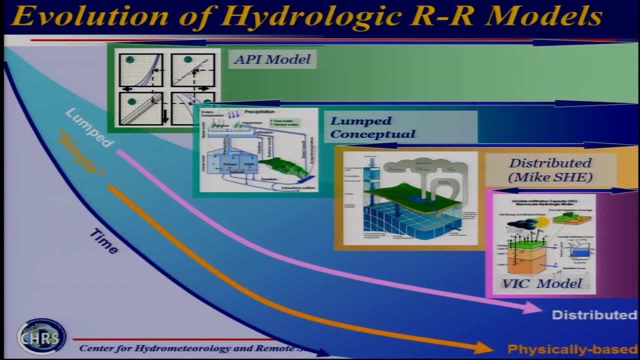 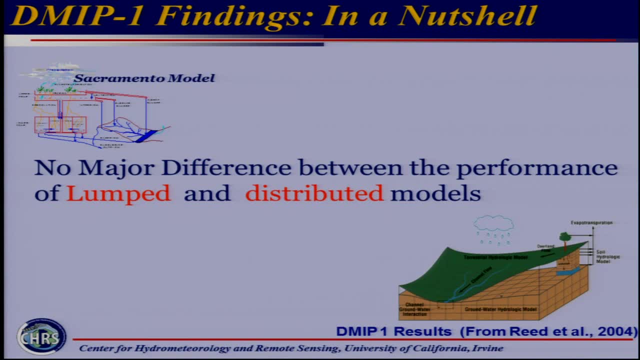 based on complex and, of course, as complexity increases, requirements also increase. So what's the message? A study was done by the National Weather Service because people who are doing a lot of developments in the distributed models complained that the Weather Service is not waking up to the realities. 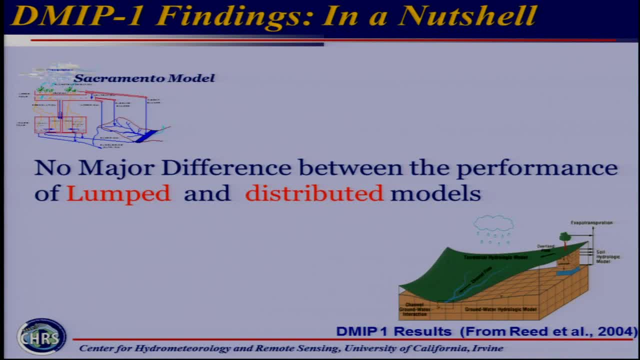 that we have more advanced tools, and why aren't they switching to more advanced tools, which are the distributed models? So they conducted a number of two or three years of in independent study and everybody who had a distributed model or a lumped model came. 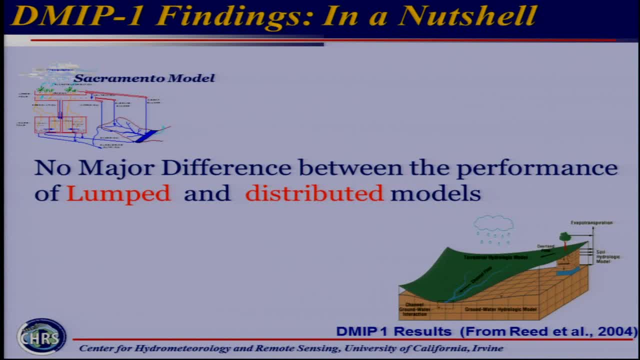 They gave you the data for a few watersheds, You run it and then they took the outputs and made a comparison and, at least on the first phase of this, it showed that there was no major difference between the performance of lumped and distributed models. 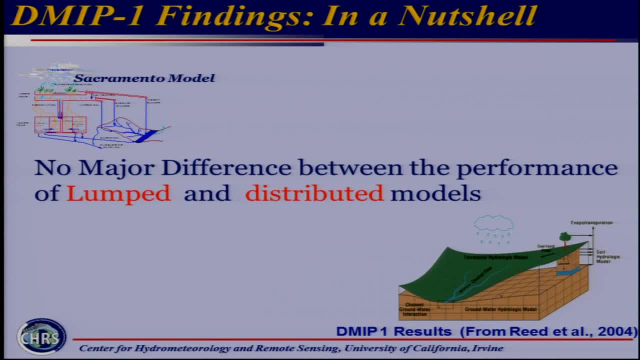 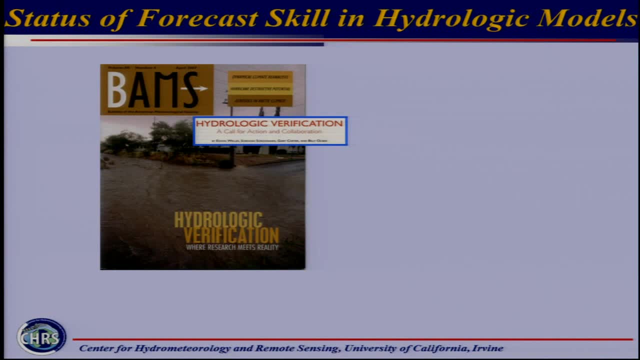 which has now redirected people to start thinking about. why is that the case? okay, Now I had a former student, Edwin Wells, and one of the things was that, well, the National Weather Service, on the hydrologic side- they never really keep track of how good their models do. 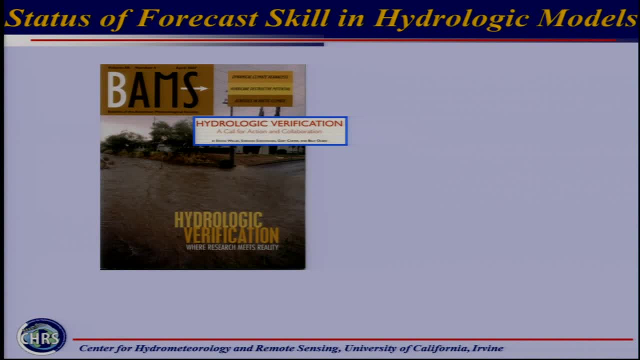 They do a forecast, they throw it out and tomorrow you won't have any trace of it, While on the weather side, they've always kept the information that they can keep- the skill of how well they predict the temperature in the next five days, for instance. 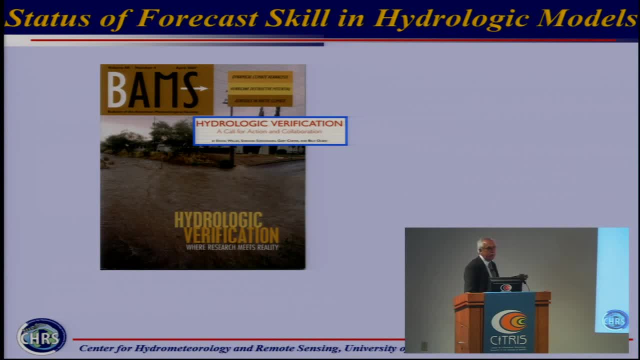 So we did. At least he was able, working for the weather service, find some data for a number of areas where they hadn't thrown out the forecast. they did, and what he did was, in fact, it was a paper that we published in BAMS. 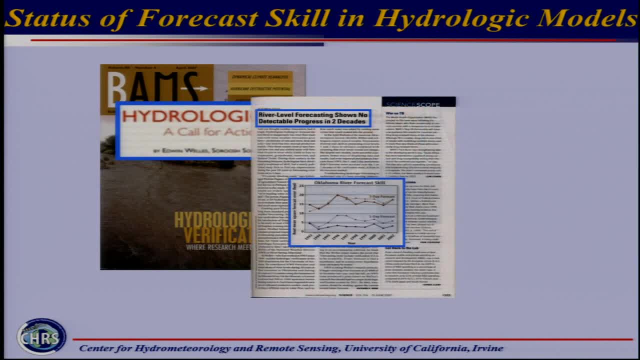 Bulletin of American Meteorological Society and in fact it was picked up by Science magazine and the title was: River Level Forecasting Shows No Detectable Progress in Two Decades that these models have been developed, And I will try to explain this. 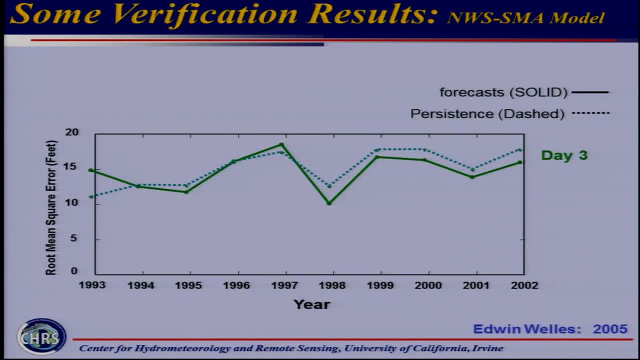 in the next diagram that the upshot of the Edwin study was that the forecasting skill of a hydrologic model is no better than just persistence after three days. So you cannot necessarily expect a model to do any better than just assuming. you know things are going to stay constant. 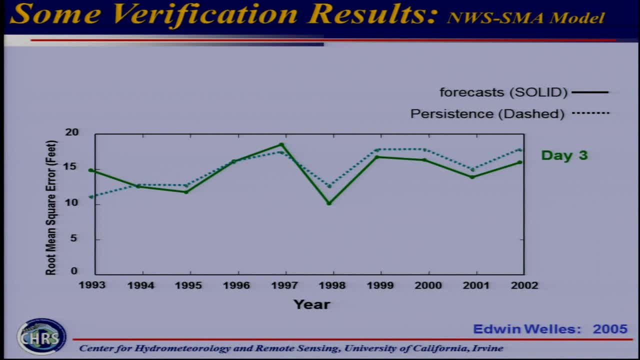 for the next three days, And there are two things about this diagram that are important. This one particular case was for I don't know which of the basins, but I think it was in the Oklahoma area. is that you expect that in the 10-year period? 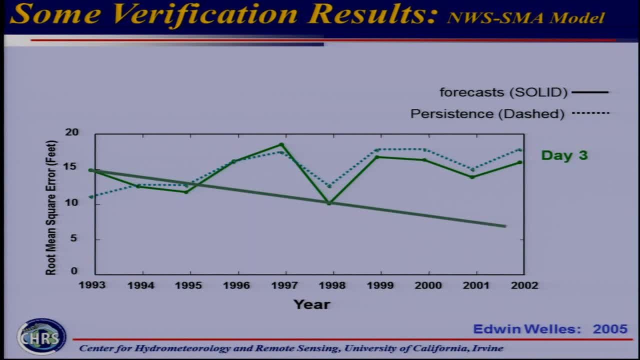 you draw down the error, but it never went down. That means that even the models that they run, they haven't really updated them and therefore you have not reduced the total amount of the error in that as compared to what you see there. okay, 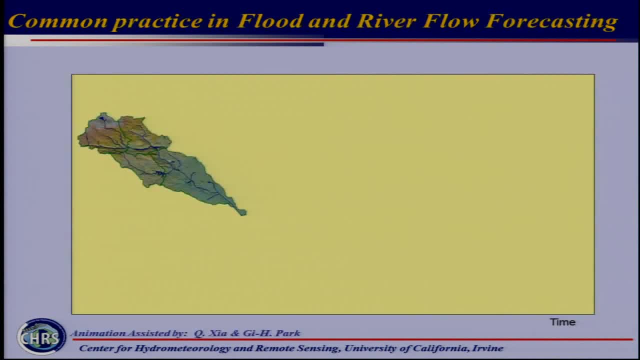 And then the skill hasn't improved. So let me just, Let me just tell you what these things do when we do a flood forecasting. So you've got a number of gauges over the basin, You may have a radar system, You may have satellites- nowadays, 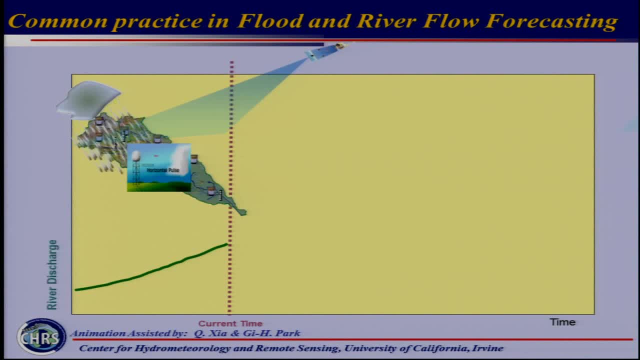 which we process precipitation information And of course, it falls over an area and this is the rain: quantitative precipitation estimates. You have to process that information And this is what it is up to the current time. Then you pick a hydrologic model. 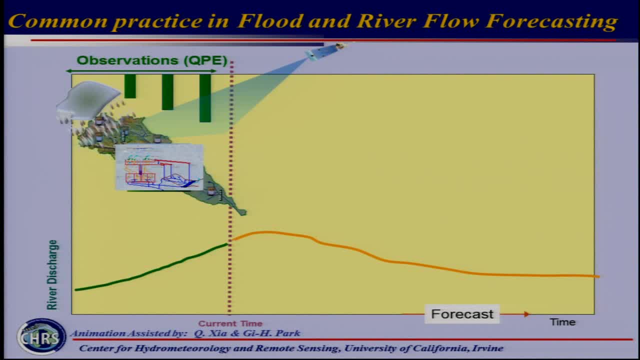 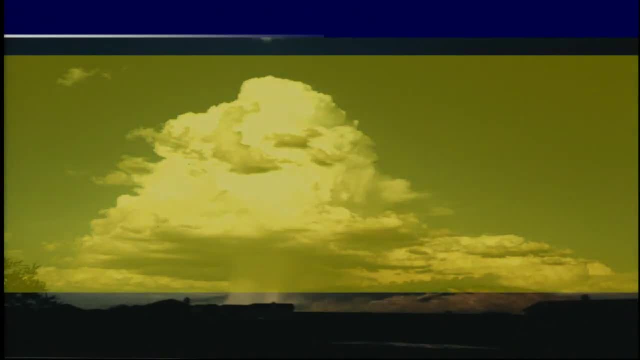 feed the rainfall into it to come up with a brownish or yellowish line here, which is the forecast into the future. okay, Now the lead time is always a question, especially with smaller watersheds. By the time you try to get a forecast, 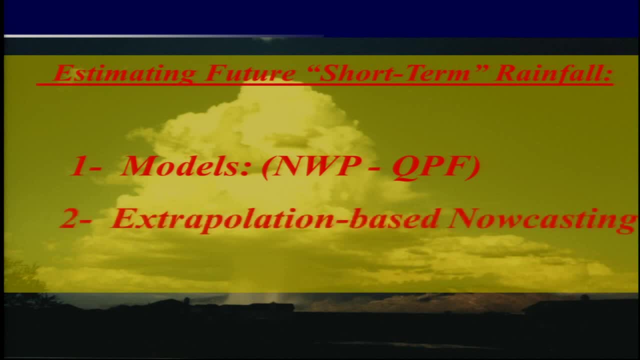 a flash flood has come and gone, and your models have been unable to do it, So for that reason the emphasis has been also put. can we predict the rainfall a few hours earlier or days earlier, And then that allows us to run it through the model? 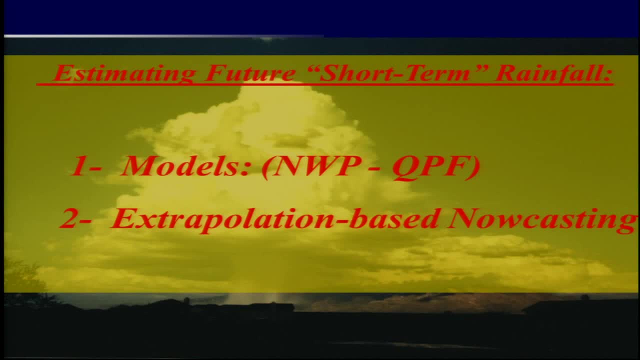 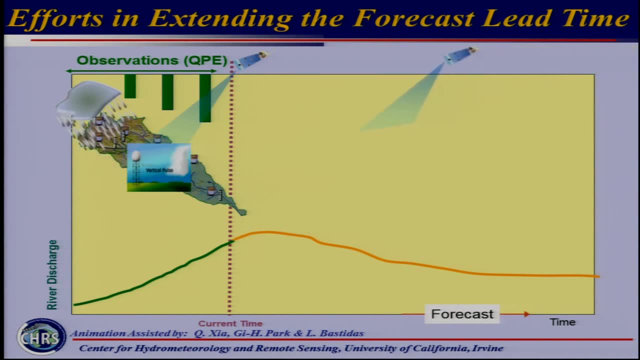 and have a better forecast, a lead time on the runoff. So there have been different techniques that have been pursued and followed, And what happens in this case- I already showed everything up to here- is that you run numerical weather prediction models, Like you do the temperature for five days. 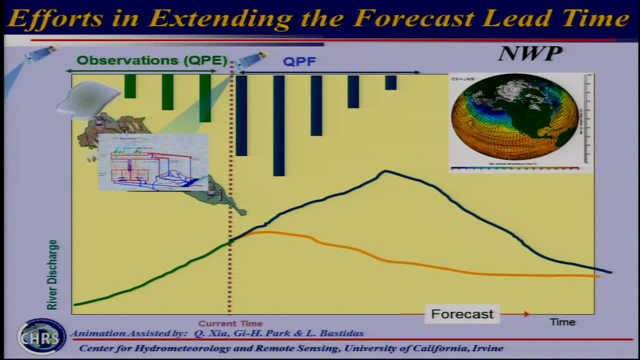 now they're trying to come up with what we call quantitative precipitation forecast estimates of rainfall into the future. okay, And there is a website, If you go. they try to provide that And the hope is that in the future we will be able to increase the lead time. 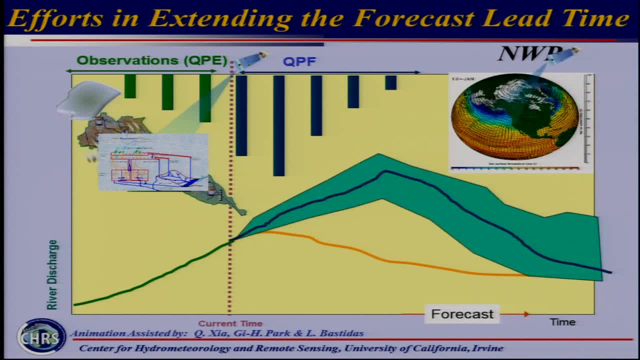 of these flood forecasts. Obviously, as you go into the future, the uncertainty bound increases and work for the scientific community has been more towards how can we reduce the amount of error? And I can't really get into that in this talk, but you know there are different ways. 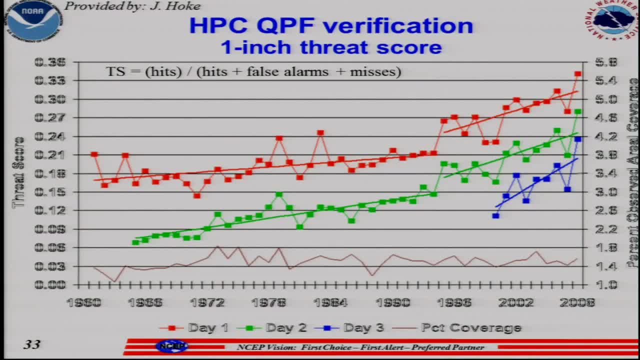 by which people are trying to pursue these things. So here we rely on numerical weather prediction models to give us better estimates of rainfall into a day in advance, two days in advance, et cetera, And this is what is known as a scale of the prediction. 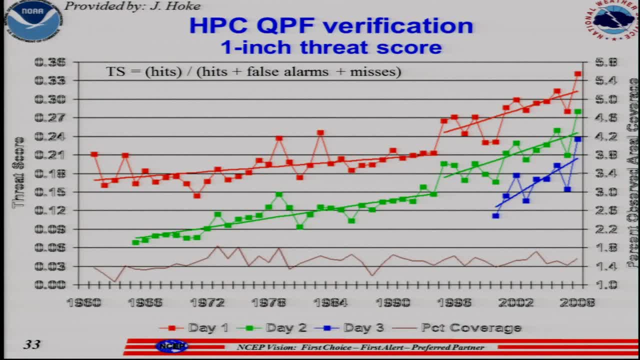 And it goes based on a scale of zero to one. okay, And when it comes to the temperature, when you see the weather forecast on TV, they give you a five-day forecast And they've become pretty good with respect to the temperature and the general idea. 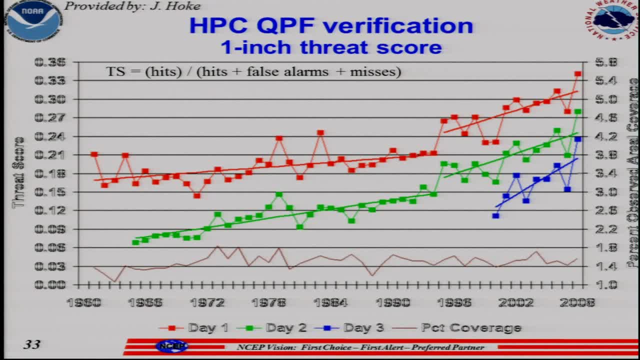 whether an area gets rainfall or not, But in terms of the magnitude and the amount, it's not really doing that great Temperature. they can actually do with a scale of about 0.7, 0.8, 0.9.. 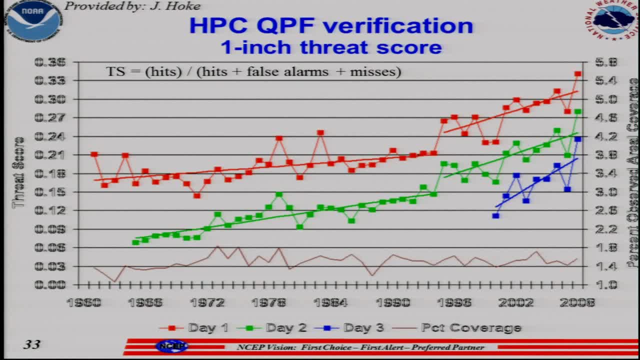 But when it comes to rainfall estimates, even at the one-day forecast ahead, the scale is still not acceptable. okay, It's in the range of 0.3 to 0.6.. And as a result, it has limitations and therefore you cannot trust it. 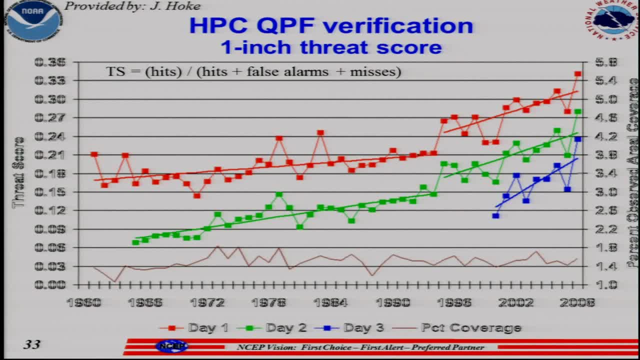 to come up with a longer. But you know, the good news is that the work that is being done is actually showing improvements And this big jump is when the numerical weather prediction model at NCEP switched to a new version, And certainly there was a quantum jump here. 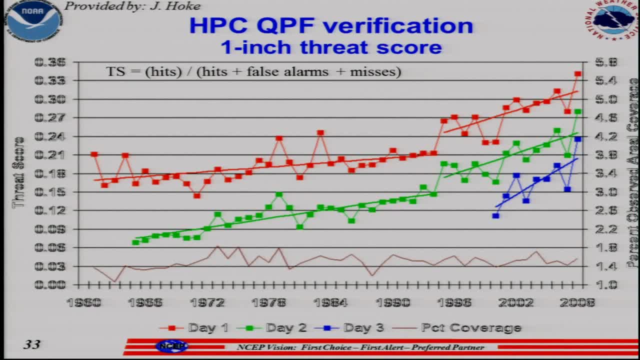 and that's also reflected in the quality of the forecast. they provide for temperatures and others. So in a way, as a hydrologist, we are also at the mercy of the meteorologists and hopefully their improvements in this area will help us improve the forecast. 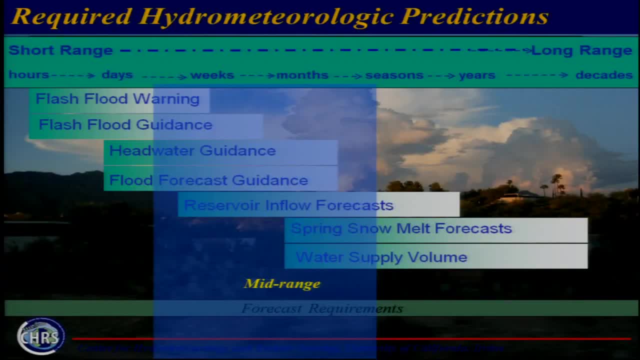 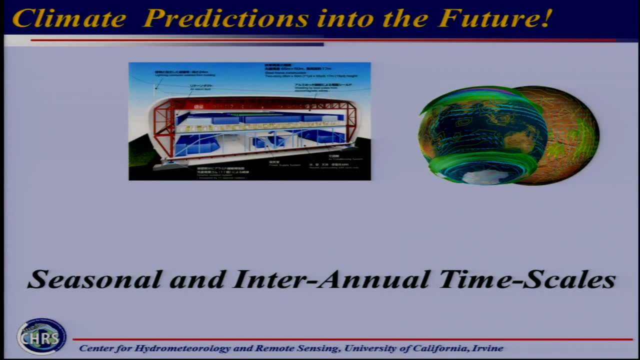 at least on a short-term basis. Let me go into the mid-range forecasts. Let me just choose an example here, And this is known as seasonal to inter-annual, and at this point I guess people run climate models in order to come up with these forecasts. 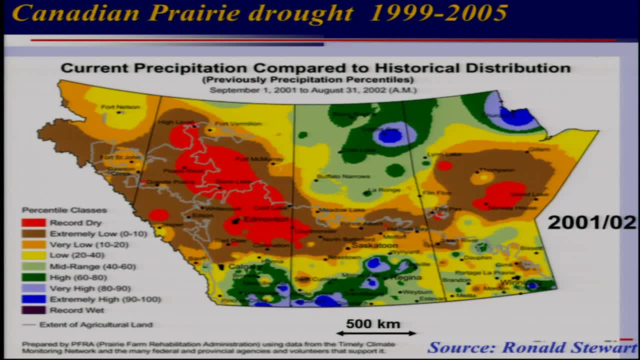 The case in point is a situation between 1999 to 2005 that really affected the Canadian prairies in this Edmonton area. So the redder the area is that extreme drought in this area that was experienced. This is the information from 2001 to 2002.. 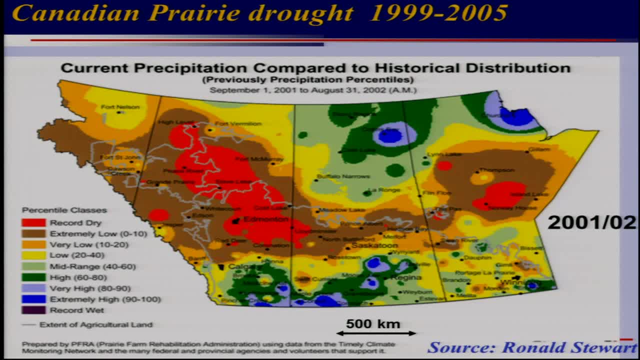 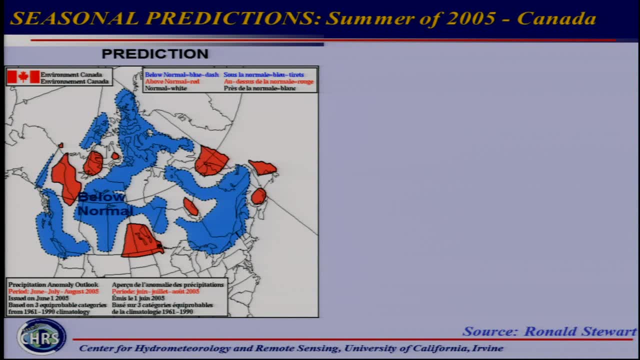 Anything that is getting red means that that area is suffering through a severe drought. So in 2005,- and it continued for three years, four years in 2005,. this is what the climate prediction at the seasonal scale was for the summer of 2005 for the same area. 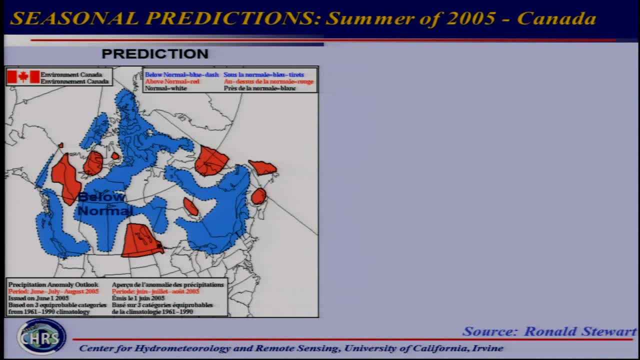 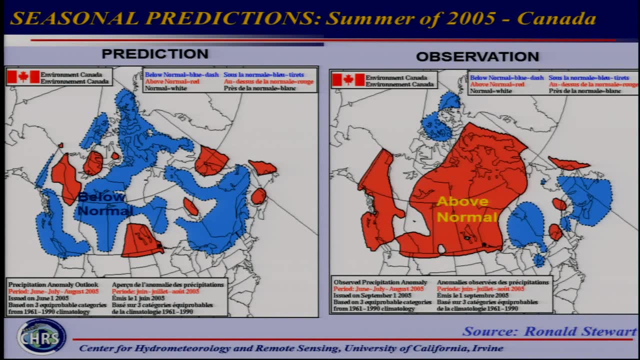 It still predicted that it's going to be below normal rainfall and the drought will continue on, And it turned out that it definitely didn't match the predictions or the climate predictions, and in fact, it turned out to be way above normal in terms of precipitation. 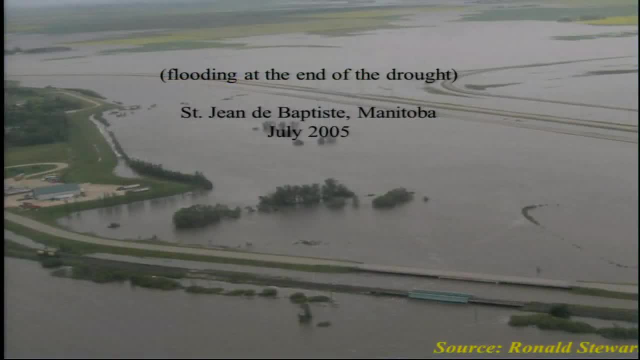 And they had some of these predictions. they had some of the worst flooding And the drought within a matter of weeks was completely gone. So the point is not to take away from how- maybe not good- the climate models, at least at the seasonal to inter-annual, are. 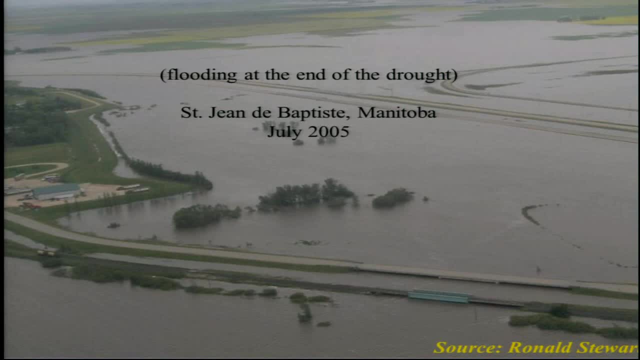 It's to point out that nature is a very tough one, And trying to really come up with models that have that kind of scale prediction is always difficult. So you have to always have a little bit of doubt with respect to what you get, And they did some studies. 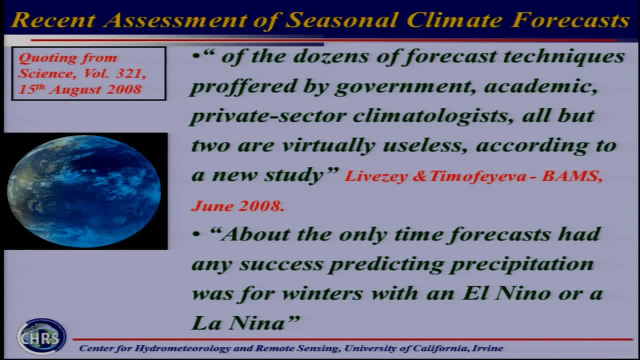 And in fact Leavesy and Temo Fiorio worked at the National Weather Service and he recently retired. He was in charge of the seasonal forecasting for the National Weather Service And, interesting enough, a paper that they wrote, studying most of these, came up with the following conclusion: 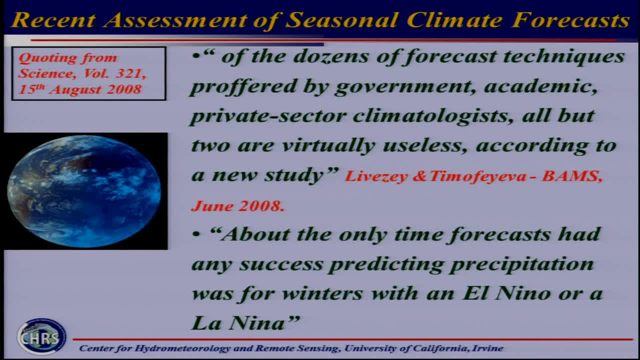 that actually was picked up by Science Magazine as well. It says: of the dozens of forecast techniques preferred by government, academia, private sector climatologists, all but two are virtually useless. Okay, And that was not necessarily a pleasant thing. 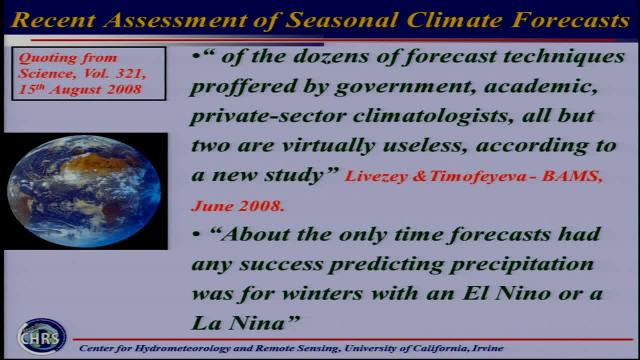 And his employers were not that happy when they published this thing. But the good thing is that his collaborator still works for the Weather Service even though he retired. But the only thing is that, even with those two models, this is about the only time forecasts. 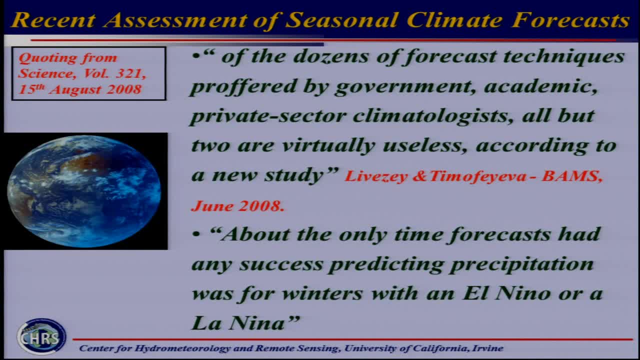 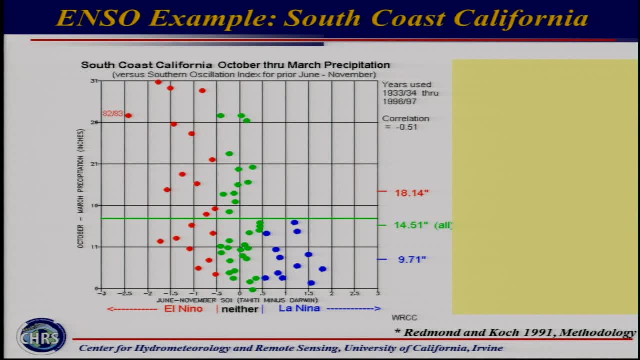 had any success predicting rainfall was winters with an El Nino or a La Nina, And if you look at California, for instance, the southern part of the state- anything that is in the range of 0.5, 0.05 minus to 0.5. 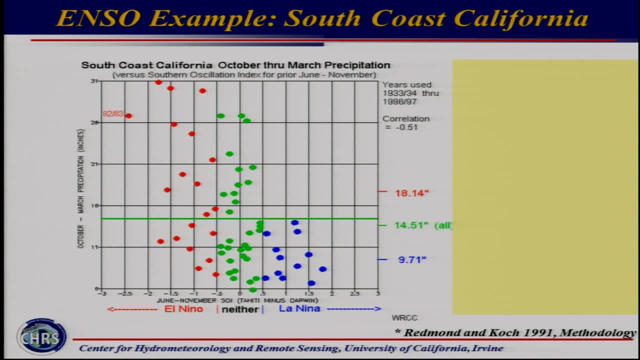 falls in the neutral zone. Anything in this case on the ENSO scale means that we have El Nino conditions And anything on that side represents the La Nina. So in general it's been recognized in the western United States that when we have El Nino, 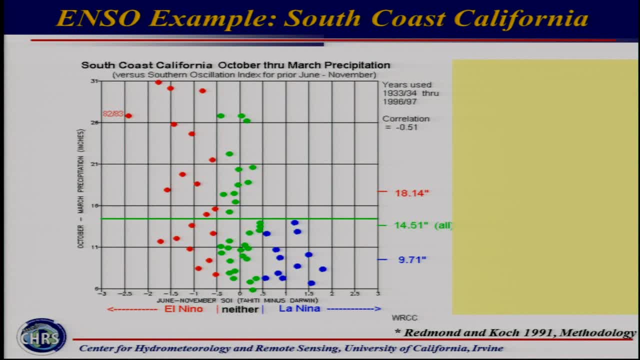 we might have wetter-than-average seasons And when we have La Nina we have drier-than-average conditions. So these are for the south coast of California And if you notice that obviously we have an El Nino winter, maybe very wet. 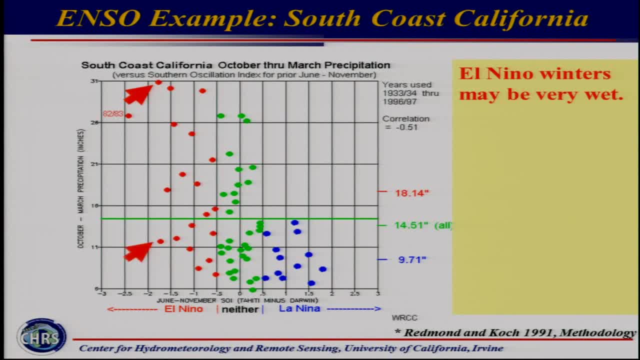 but there have been El Nino years that have not been wet at all. Okay, And the second thing that you might notice is that very wet winters are typically El Nino. That's what is expected, But not always We've had neutral years. 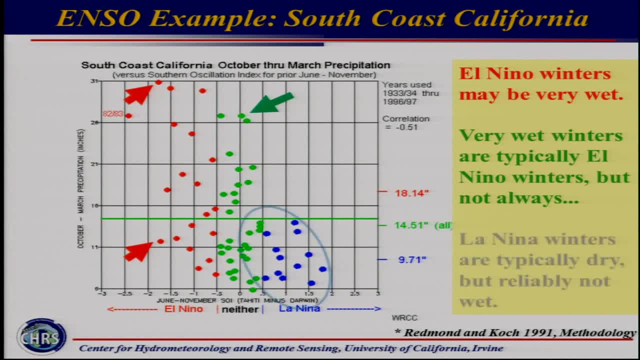 where we've had very wet years. Okay, And last but not least, is that La Nina winters for at least southern part of the state, are typically dry, but reliably not wet, meaning that there's still uncertainties, but at least all the blue points that you see. 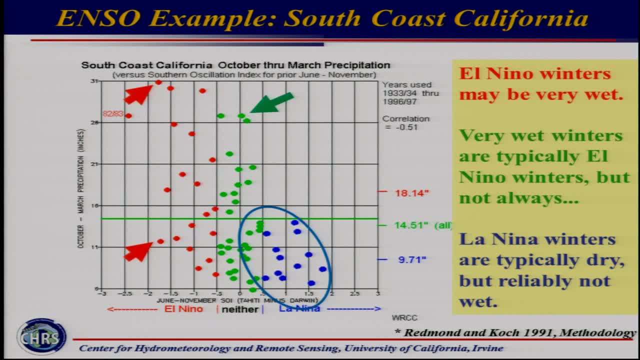 happen to be La Nina years and they're pretty much clustered in this area. Okay, So again quite a bit of uncertainties exist, and that affects people who are in the planning business for water resources, et cetera. I come and take. 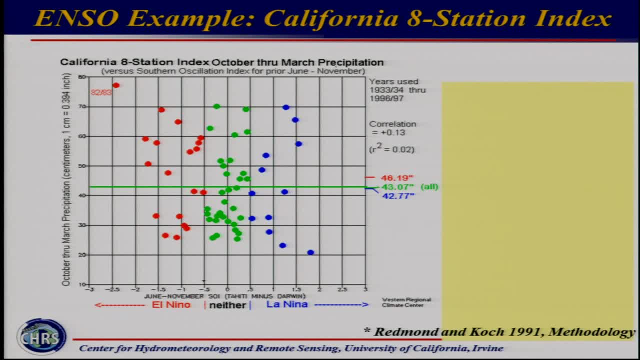 These are known as the A8 Station Index and I think these represent the northern part of the state Norm. you may know about them. I think it's in the Sierras, So you see, the data is a lot more scattered in this case. 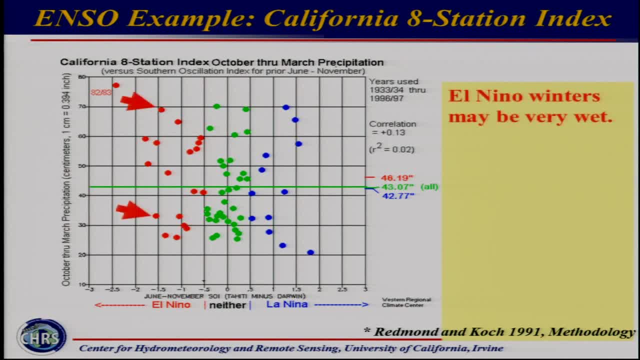 So again, if I do the same kind of examination, I do have El Nino years that are pretty wet, but I also have El Nino years that are not necessarily wet, And the same goes here In the neutral zone. again I have had years. 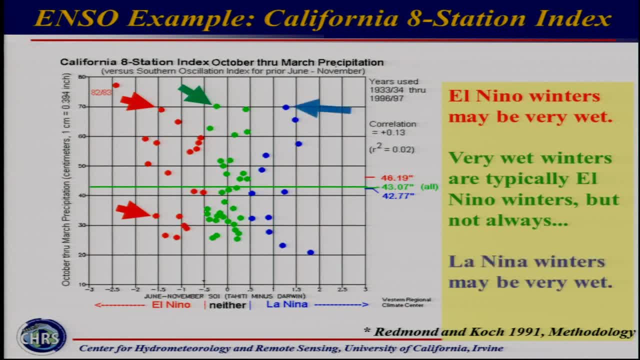 that have had quite a bit of precipitation, And then, in this case, when you come to the northern part as opposed to the southern part and even Arizona, that La Nina winters are even more uncertain. You know, we've had La Nina years. 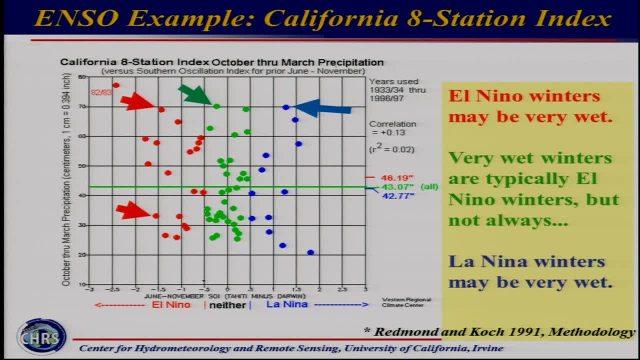 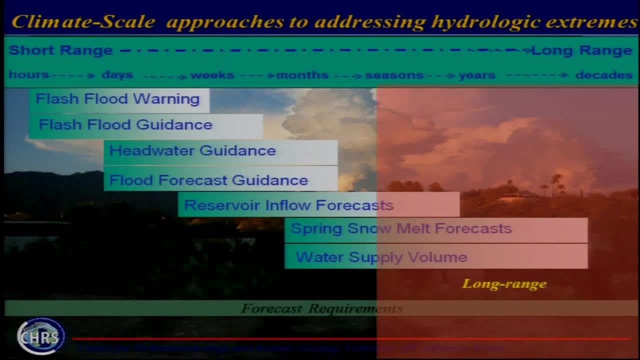 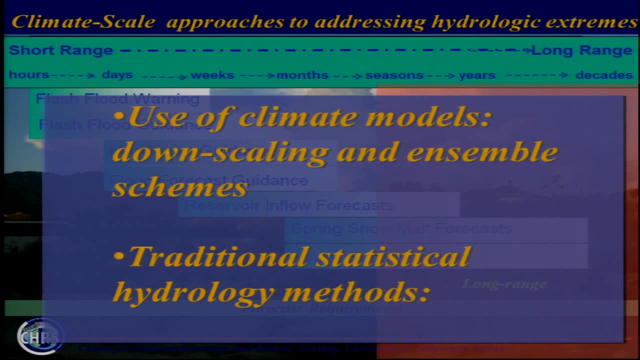 that have been pretty wet, while in the previous case I showed you they were all clustered around not being relatively wet. Let me now move on to my last part of this presentation, which is the longer-range forecasting At this point, the use of climate models. 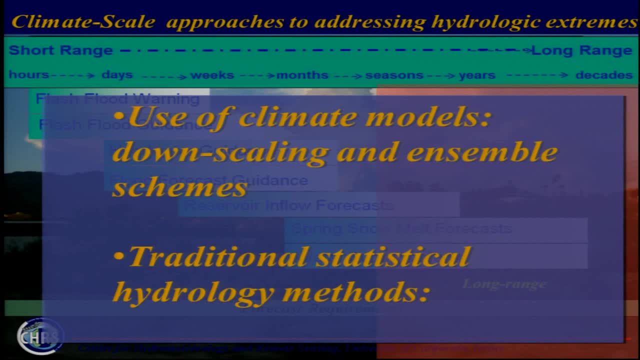 has been extensive. People use them for different types of downscaling to regions. You know the global models so you want to do California. you better take the grid area or an area and then try to downscale it and use the regional models. 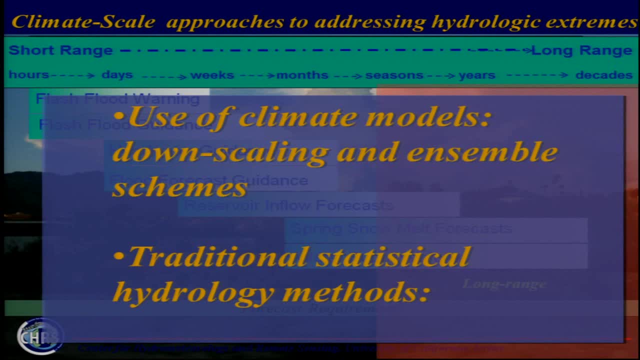 in order to see what the consequences of the climate scenarios are, say for California or someplace else, And then also in the old days, we used to use what is known as traditional statistical hydrology methods, and I'd like to talk about those. 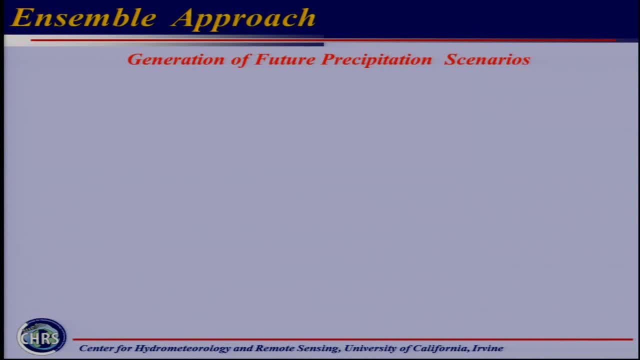 So generation of future precipitation scenarios are what a water resources person would be interested most. Okay, So what happens is that in an ensemble approach, you may choose multiple number of models, different models, and everybody's been doing that as one way to do it. 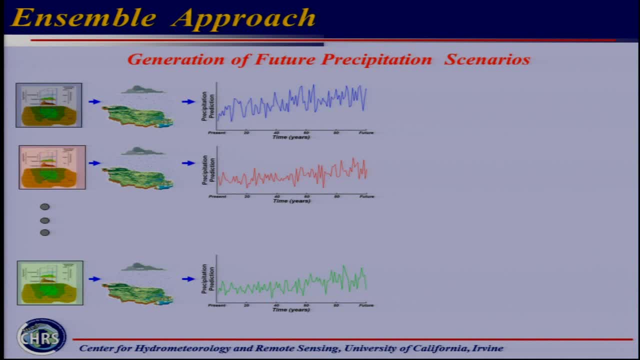 And each of the models based on initialization that you do and downscale to a region. you generate various scenarios of precipitation rainfall from these models and you get them all together and create an ensemble, come up with an ensemble estimate of rainfall into the future. 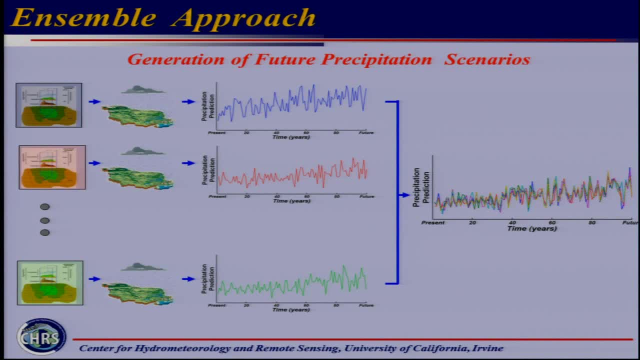 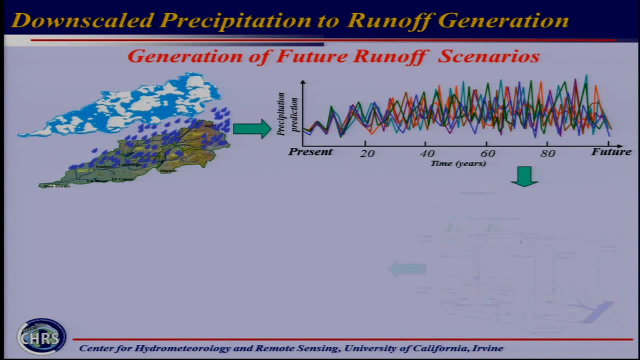 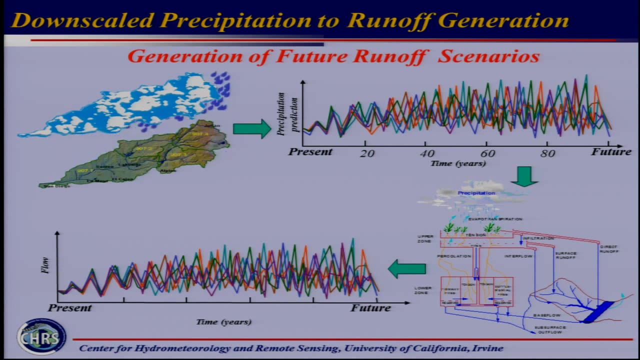 maybe 20,, 30,, 40 years into the future. Okay, And then, using those ensembles, you feed them into a hydrologic model, if your interest is looking at the implications from a hydrologic cycle point of view and generate different scenarios of runoff. 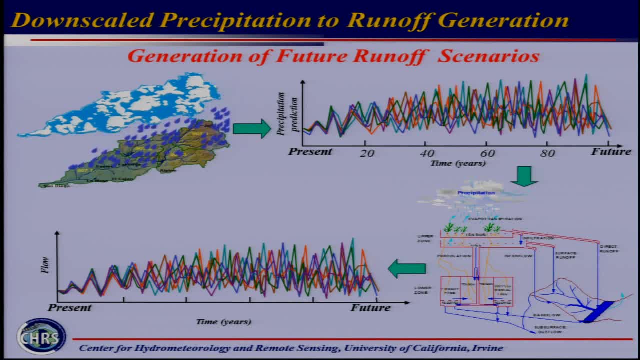 for your favorite river. Okay, And then use these scenarios of runoff in order to decide what would be some of the areas or consequences and what should be the amount of resiliency that you may want to have in the system if, unfortunately, you have years of sustained drought. 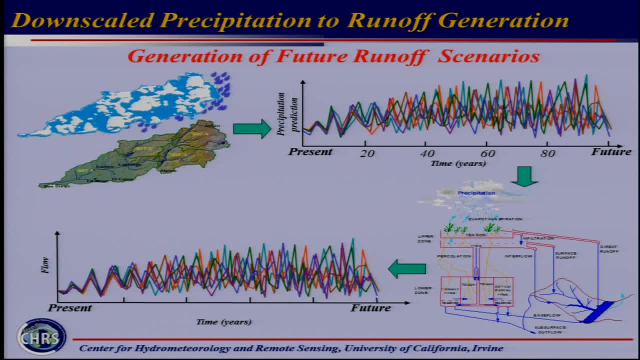 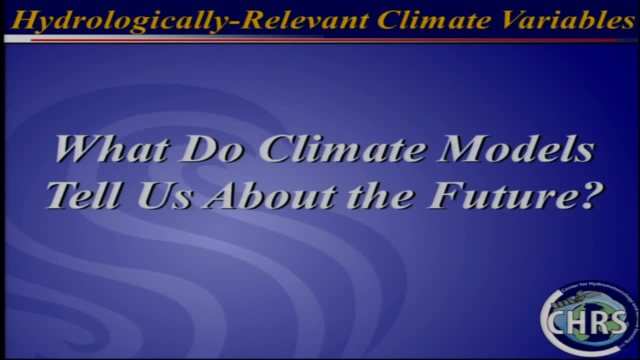 then where would you get the water from? So these are the type of things people use in water resources planning in order to decide the future. So what do climate models tell us about the future? Okay, well, let me just use this diagram. 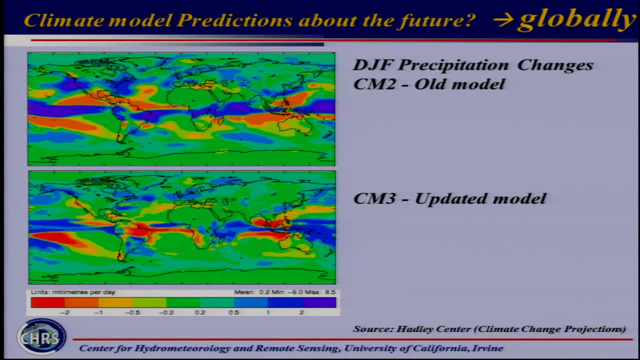 This is two versions of the CM3, the Hadley model, the old version and the updated version. And if you look, even one model when it was improved, there are regions of the world that, in fact, it completely changed signals. 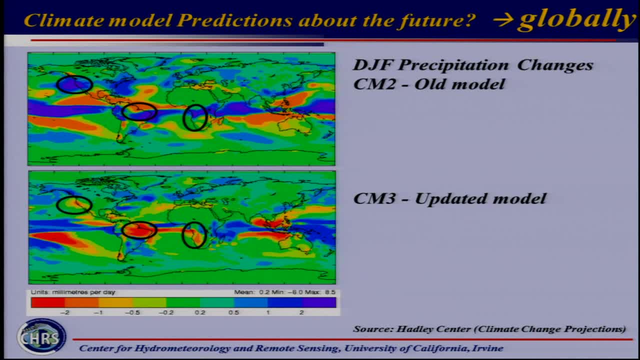 where in the older version of CM2, it showed that western United States was getting wetter. with the newer version of it, with improved okay physics in it resolution, it showed that this area is getting drier, And the same goes for a number of other areas. 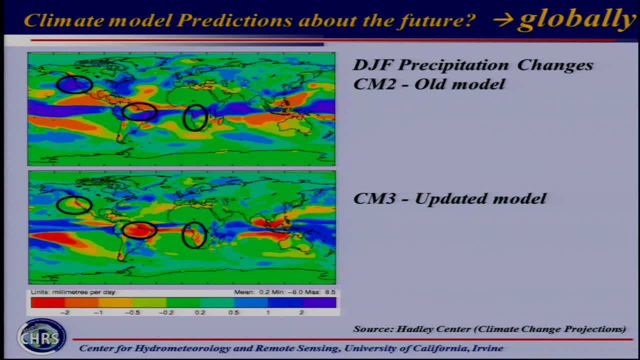 that I've identified And, given that kind of uncertainty, unfortunately they have impact on regional outcomes. And so, if you're a water resources manager, what do you do? Which one do you want to trust? Okay, it becomes whether you expect. 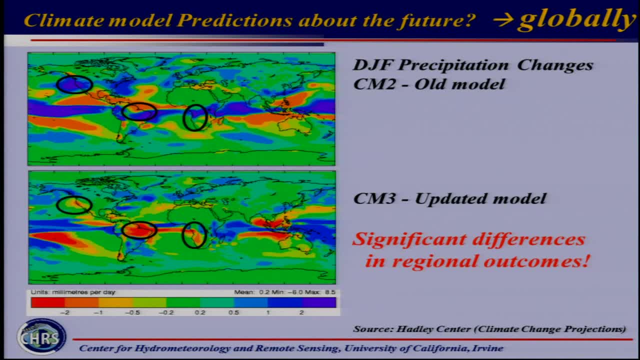 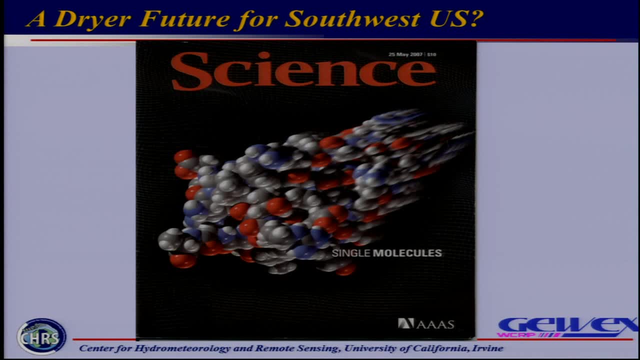 that 30 years is going to get wetter or drier. So these are the difficulties we experience with these kinds of models. In 2007,, there was a seminal paper that appeared in Science magazine And you know, Sager was the first author. 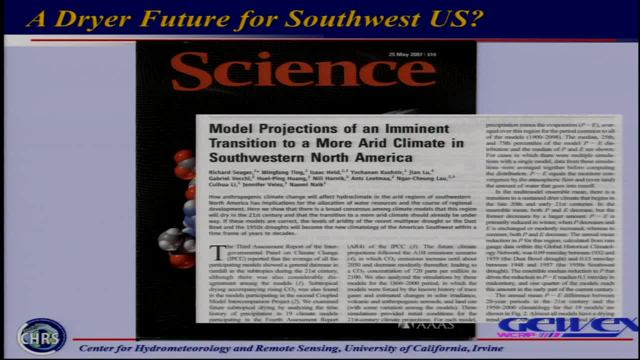 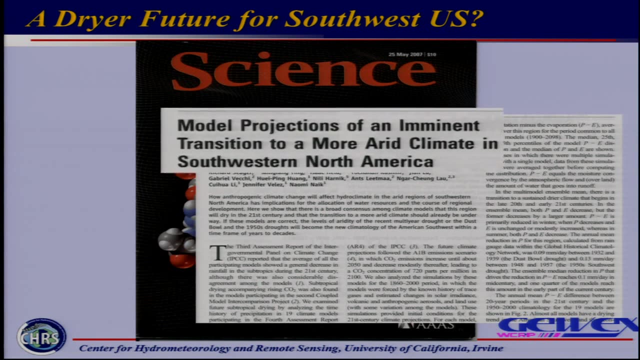 and a good number of well-known colleagues from GFDL and others were involved, And it essentially came up with this title that Model Projections of an Imminent Transition to More Arid Climate in Southwest North America. Okay, And that's really pretty profound. 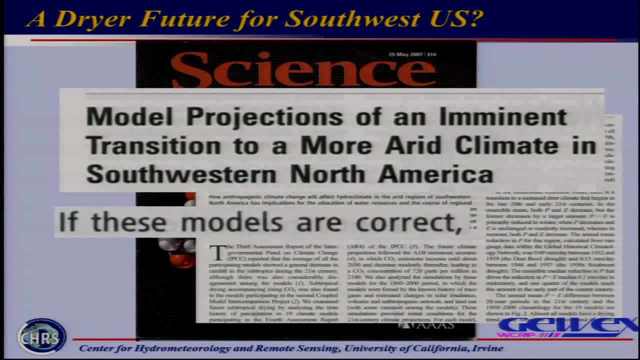 I got a call from a news person in Orange County said: what do you think? I hadn't even seen the paper, so I wanted to read it. It's really interesting. even in the abstract of the paper, it does say this: 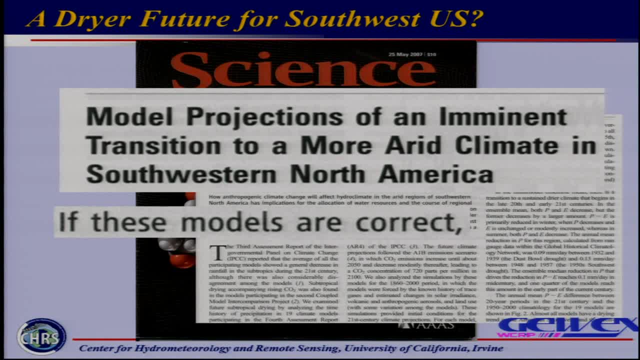 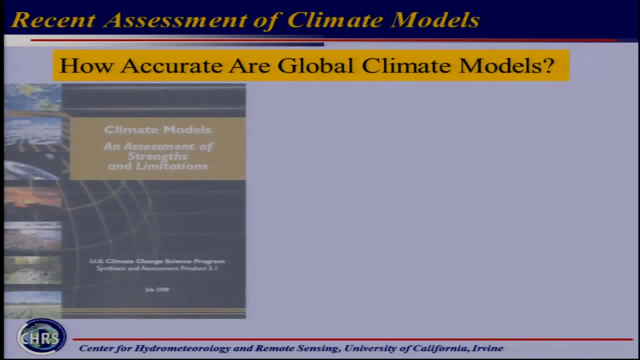 It says: if these models are correct, well, you know, that's really the million-dollar question. It really puts more doubt on this, And I'm not blaming the authors. It's just the best that they had at their disposal to try to come up with these kind of conclusions. 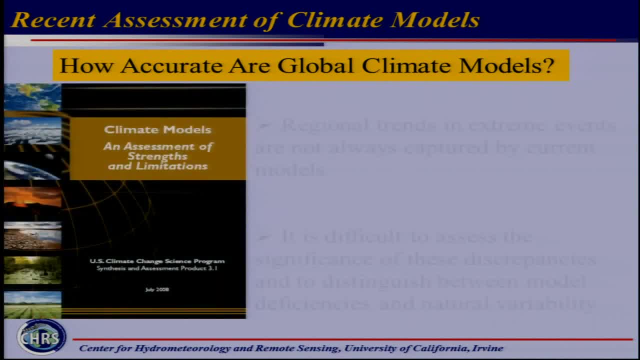 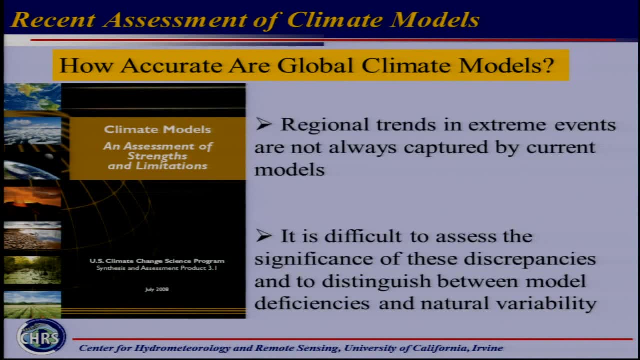 Then, as you know, US did a number of what they call synthesis analysis: 23 reports. If you go on the USGRP website, you will see that they did an assessment of various aspects of the climate over the United States. 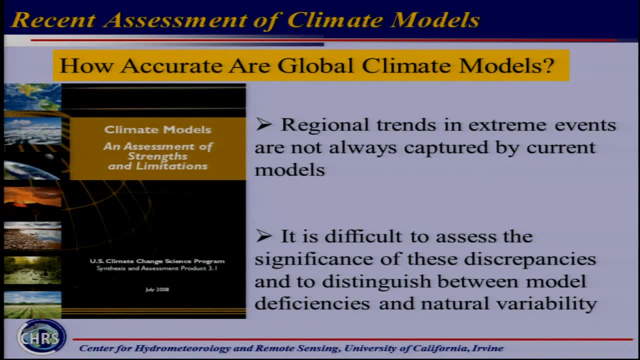 And this one was in July 2008.. This particular section was published by the responsibility of the Department of Energy, And I had the pleasure of being the chair of the final products review team and trying to get consensus from different people with even every line of the conclusions of this report. 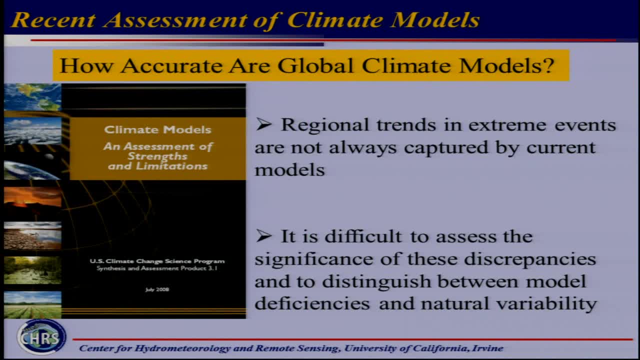 But it was published and it's available And this is dealing with the larger scale climate models And it says regional trends in extreme events are not always captured by current models. That was sort of sort of a consensus statement, very politically correctly written. 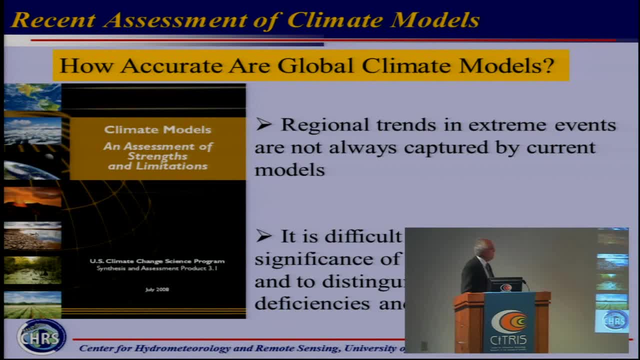 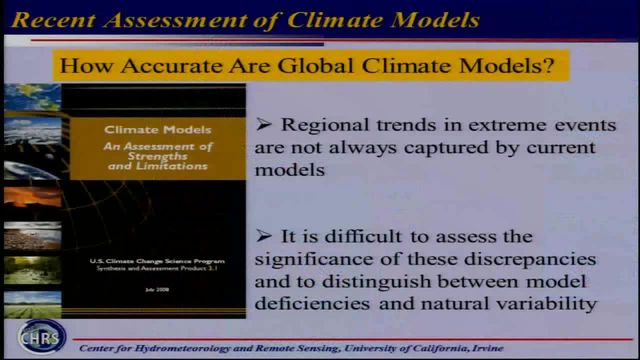 essentially saying that maybe we don't have that kind of skill in capturing extreme events, And the second part of the conclusion that I have extracted for this talk is that it is difficult to assess the significance of these discrepancies and to distinguish between model deficiencies and natural variability. 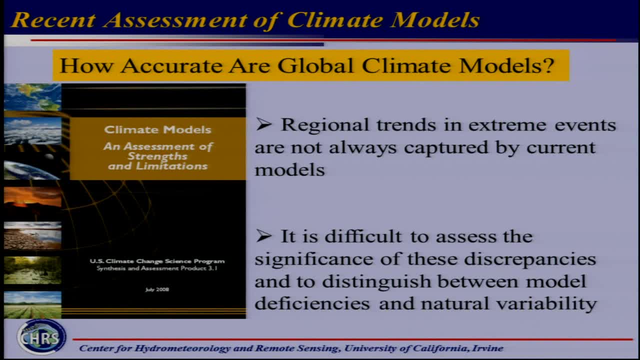 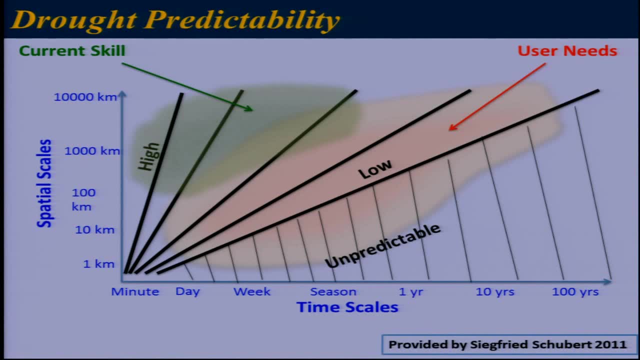 So essentially saying it's still not really fully developed to the extent that people take these things and use them for application purposes. A recent workshop we had in Barcelona, Siegfried Schubert, who works for NASA's modeling group. we came up as a result of that meeting. 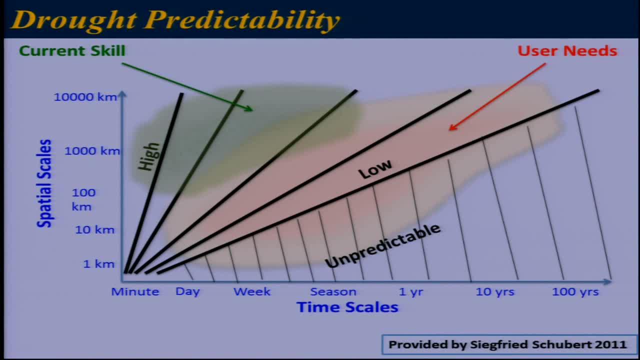 with a diagram that really tries to give some meaning to the capabilities at the present time with climate models to predict droughts. So this represents the number of years into the future and this is the size of the area that you can do. your Models seem to be okay in this zone. 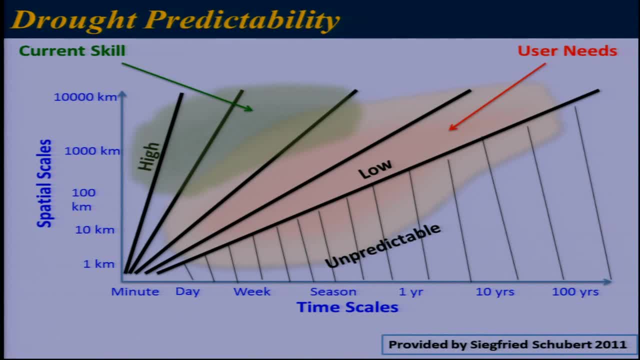 which really is on a shorter time scale, but very, very large areas of hundreds of tens of thousands of kilometers. But most regional people problems in California, Southern California, Texas. you really fall within this range of where people's interests are and unfortunately, 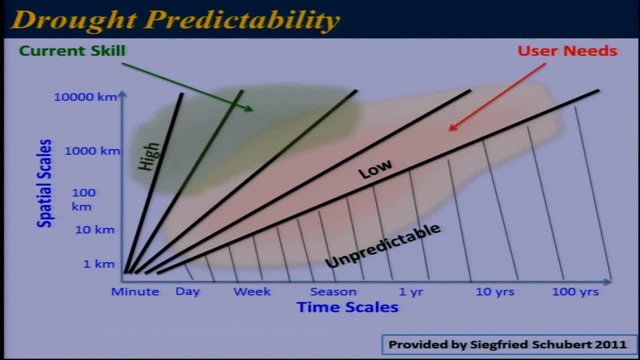 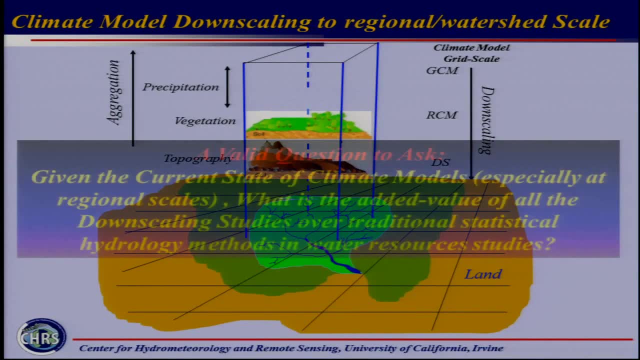 as you can see from this diagram, there was a consensus diagram that came out that the capability to predict droughts is not there yet, And so there's a lot of work to be done. okay, So let me kind of summarize here by saying that a valid question to ask. 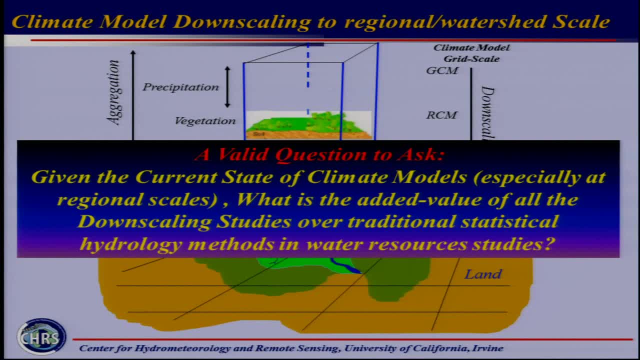 is, given that the state of climate models, especially at the regional scales? what is the added value of all the downscaling studies over traditional statistical hydrologic methods which unfortunately may have been forgotten because we've got these newer tools in water resources planning? 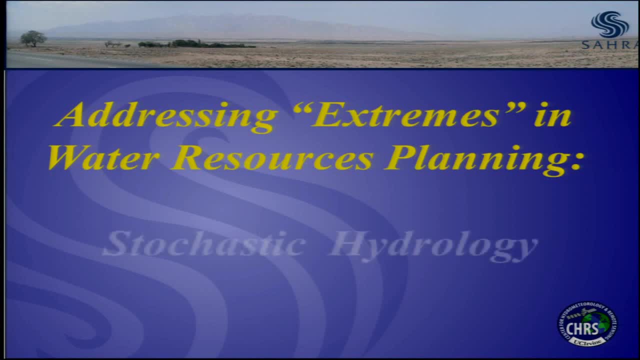 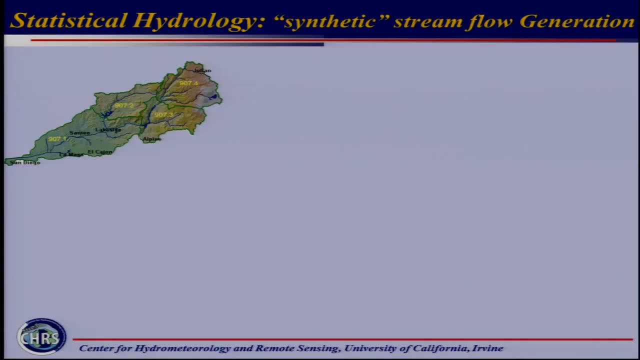 And what I mean by that is essentially the use of the good old stochastic hydrology methods, okay, And if you recall- and let me just explain this- that if I had a basin, okay, and I had a gauging station, 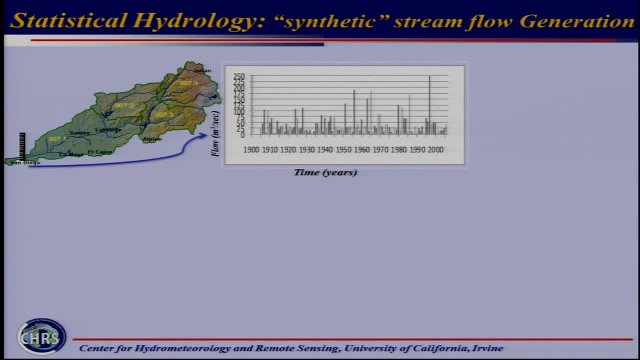 and I had go to US Geological Survey records and pick up all the runoff data from that particular gauging station on a monthly or annual basis and use the old statistical approaches that have been done in hydrology. is that above a certain threshold? 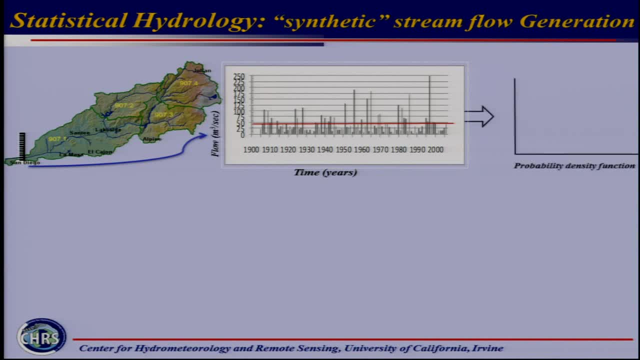 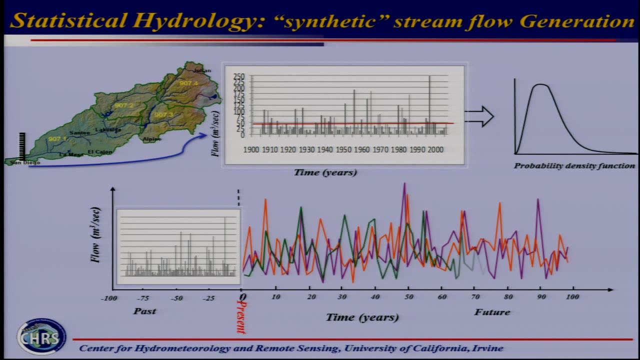 you consider these to be extreme events and try to fit a probability distribution to that part of the data, okay, and use the statistics of that. whatever distribution you fit and assume nature repeats itself and that's where, in statistical hydrology, the weakness has been that we assume nature is stationary. 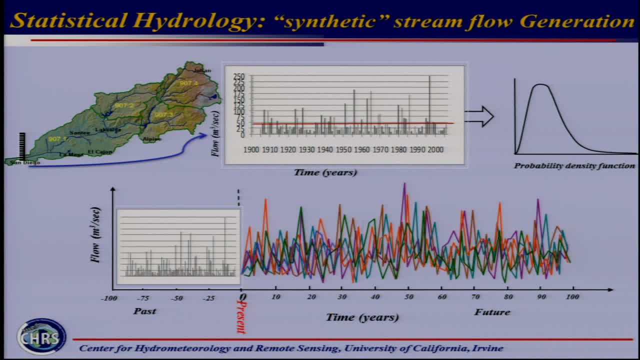 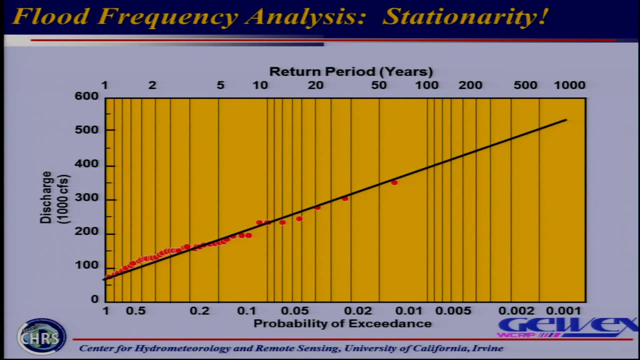 or the stationality, and it repeats itself. Then you can generate a whole sequence of runoff from this basin and again do the same thing that, as I showed before, with climate models, okay, And the traditional ways by which statistical hydrology has been done. 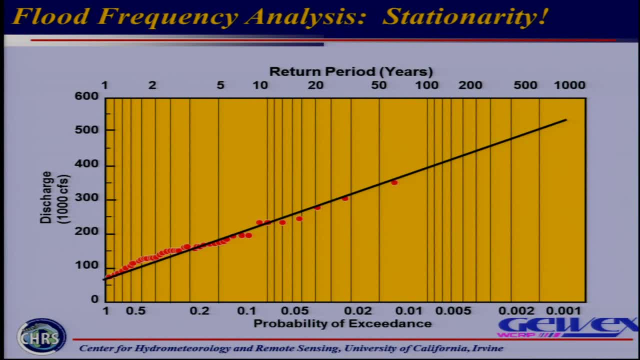 is you've logged. Pearson Type 3 has been pretty much universal. It's been used in the US and every place else in the world has adapted it because that shows that it's the best distribution to represent extreme hydrologic events. So you know, you put your data on a log paper. 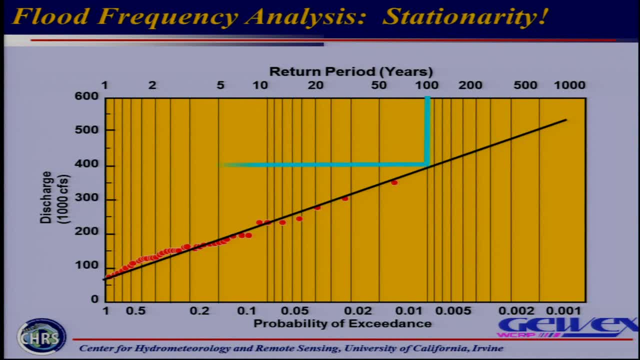 a Pearson log paper and, if you are interested, once your data is lined up, if you're interested in a 100-year flood that probably a lot of you have heard about, because a lot of design criteria and insurance et cetera are based on that. 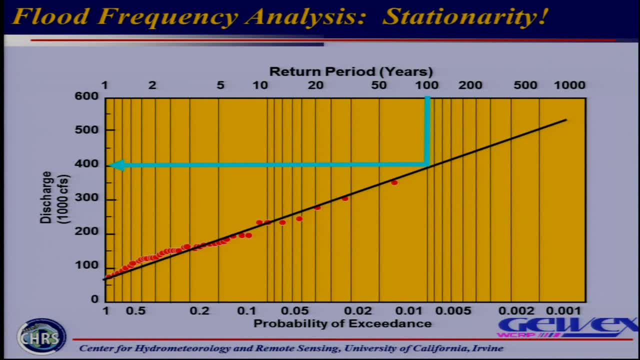 You go on this curve, come here and say, okay. for my area that means 400,000 cubic feet per second. for instance, represents the definition of 100-year flood and anything above that could be the criteria by which whether you can build your house. 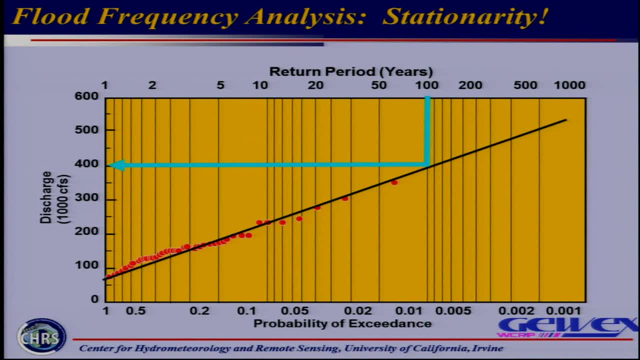 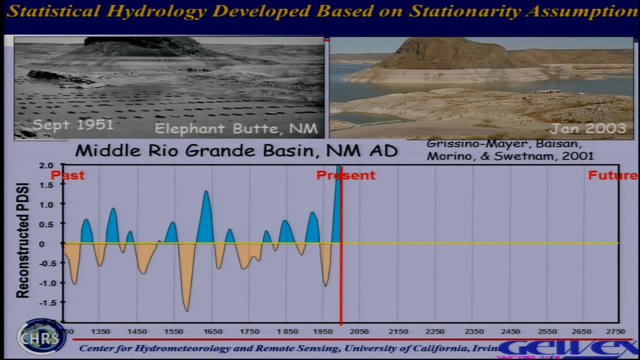 and whether you need to have flood insurance and whatnot. okay. So if that's the case, using these methods again, this is the past and you assume stationarity into the future, because that's the way it's been used, But with concerns about climate change. 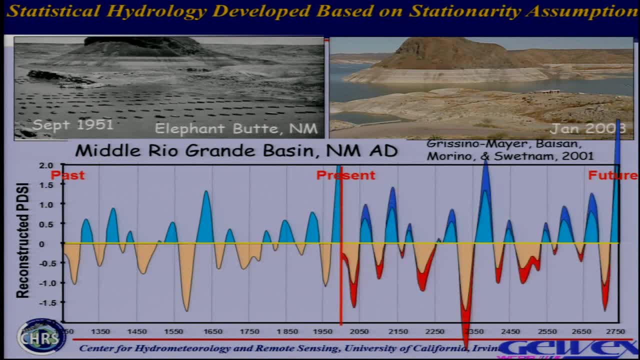 and the impact on that. obviously it may not be the right assumption. okay, That stationarity has to be considered, not a valid assumption? okay, So the question is: can you really modify these methods? And unfortunately, research in this particular field has dried up. 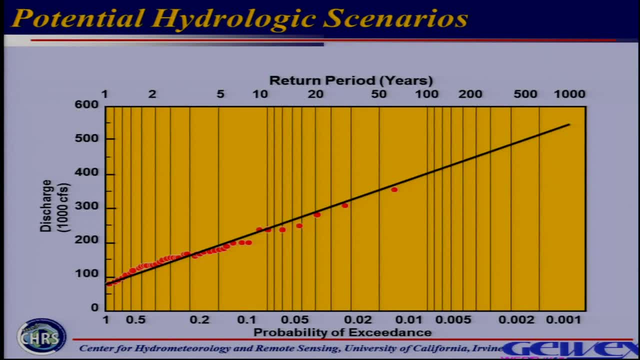 and not many people are paying much attention to it. Why is it important If I assume this curve is good forever for me? but you know climate has shifted, maybe the mean of the precipitation has increased or decreased. So by my using that original line, 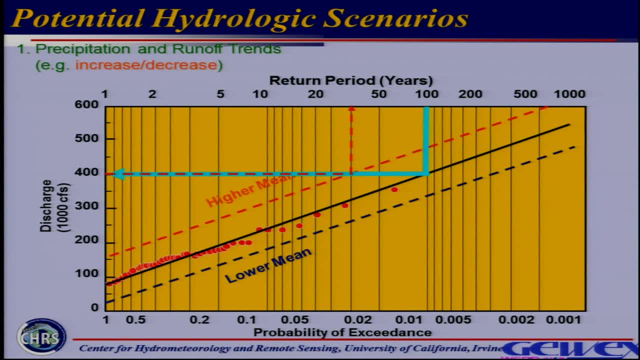 okay, I might be missing in terms of my estimates of how frequently some of these events, the same event, is happening. if, in fact, the mean is higher, that 400,000 cubic feet per second is no longer a 100-year storm. 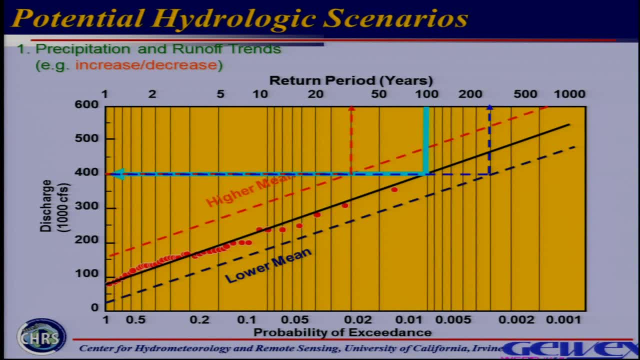 It happens more frequently, And just the opposite is, of course. if my rainfall has gone down, you know the trends have been downward, that in fact it might become much more of an extreme in the future, that it could happen once every 500 years, etc. 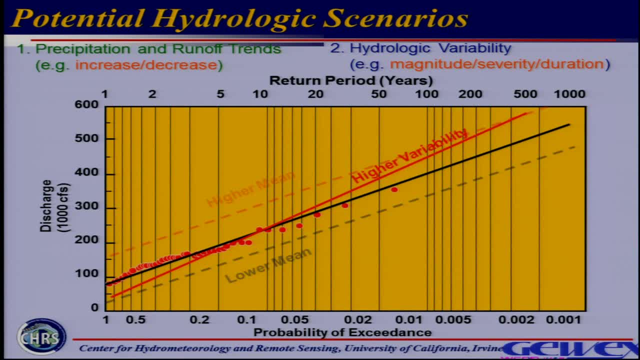 More relevant is that when we have more variability, that has been really assumed in rainfall patterns. So over a mean I may have more, higher variability or lower variability. In that case, the same thing can be argued that if I assume the same curve. 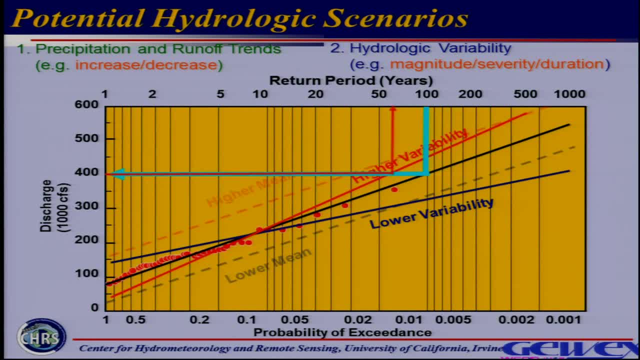 I might miss the frequency by which my storm could cause damage vis-à-vis if it's higher variability or lower variability. So these variations become really important in terms of everything we do. All the floodplain mapping that is done over the United States still goes based on the assumptions. 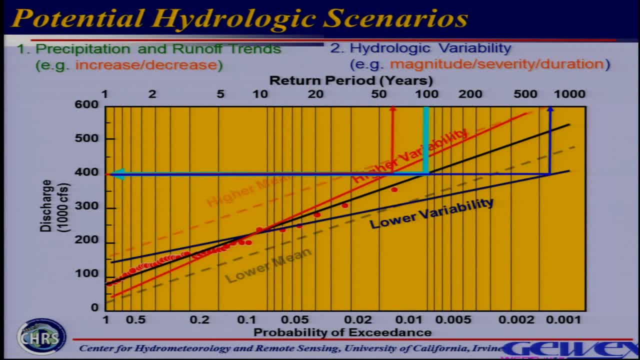 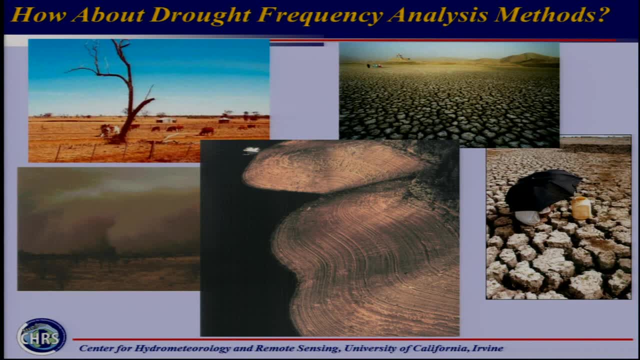 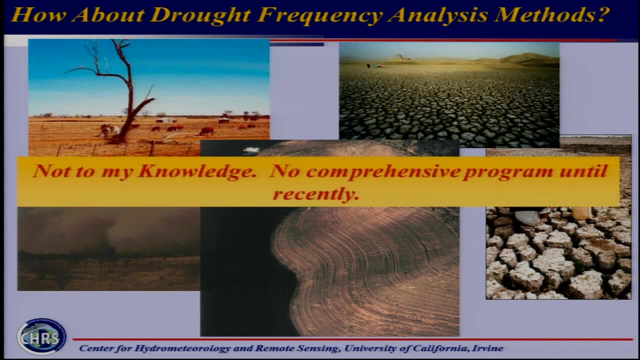 of stationarity and the same kind of data that is being used, And so that's for the flood part of it. From the drought point of view, there has never been a drought frequency analysis that I know of, And unfortunately it's just. 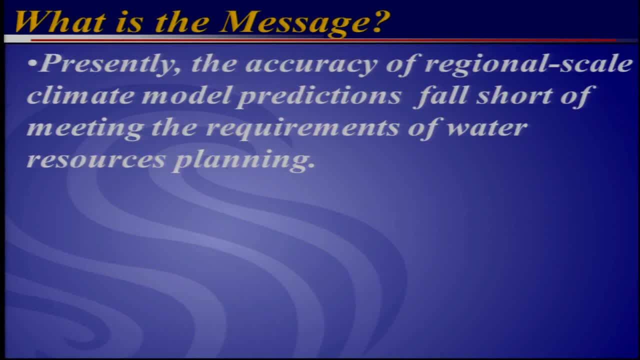 just missing. There is no statistical method. that has been done. Part of it is because we don't have the record. So let me sort of summarize here What is my message is that presently, the accuracy of regional scale climate predictions falls short of meeting the requirements. 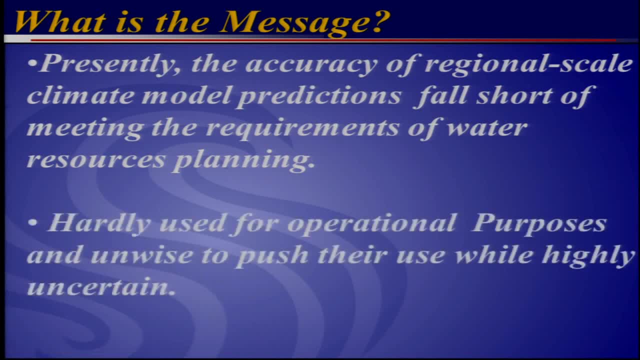 of the water resources planning And hardly used for operational purposes. If somebody tells you they're using it, I'd really like to see the evidence of it, And it's pretty unwise to push their use while they're highly uncertain. Okay, 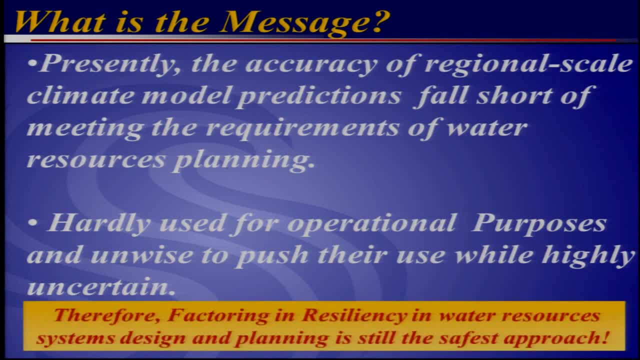 And therefore factoring in resiliency in water resources system design and planning is still a safe approach. Of course, resiliency means cost and money And I know, with the economic situations, I don't know how you can do it. 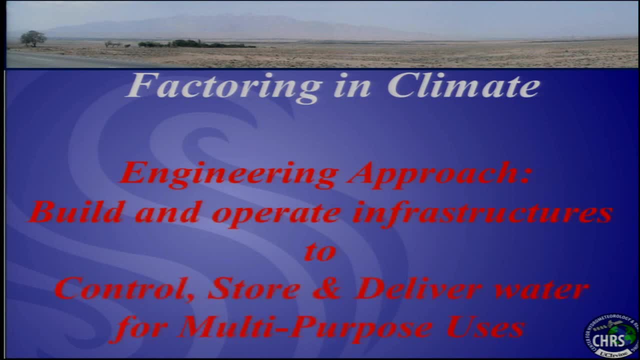 So we go back to what is known as the traditional engineering approach, which is really appropriate since I'm at Berkeley, which is well known for its engineering, And build and operate infrastructures to control, store and deliver water for multi-purpose uses. 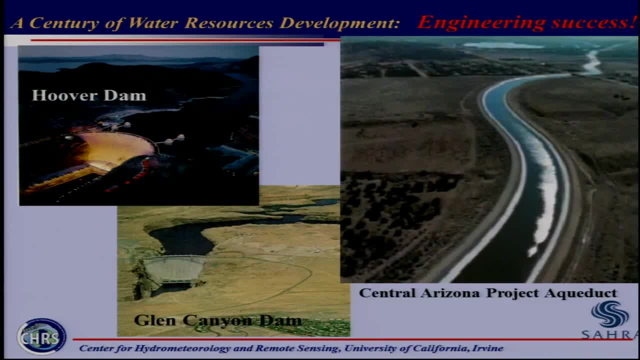 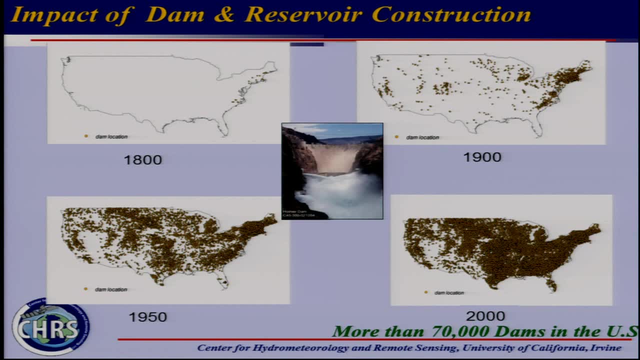 Okay, So we see evidence of that And US is quite well developed in terms of the infrastructure. If you look at the history of dam building in the US starting from the 1800 to 1900, 1950, 2000,. 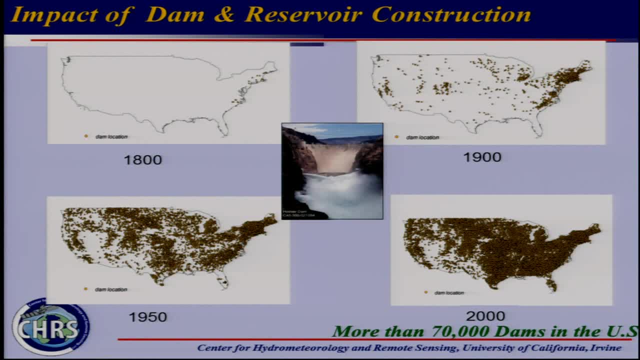 we don't build any more dams, But more than 70,000 dams. Some of them have been built in the US, some of them being decommissioned because of not being safe. And if you think we have a lot of dams. 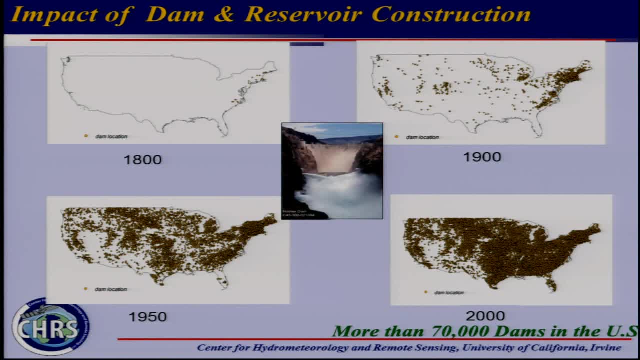 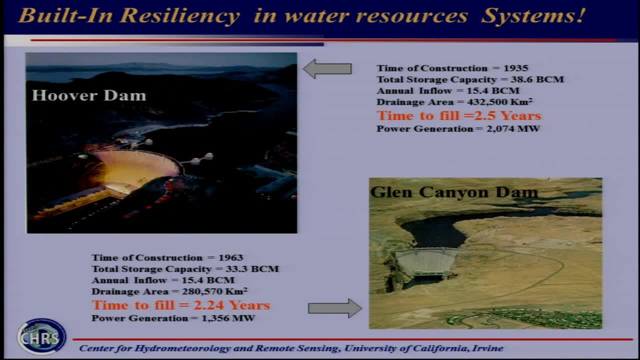 the same standards apply to China. They have now about close to 80,000, 85,000 dams in China And it's really impressive. So when I talk about resiliency, if you look at these two dams on the Colorado River, 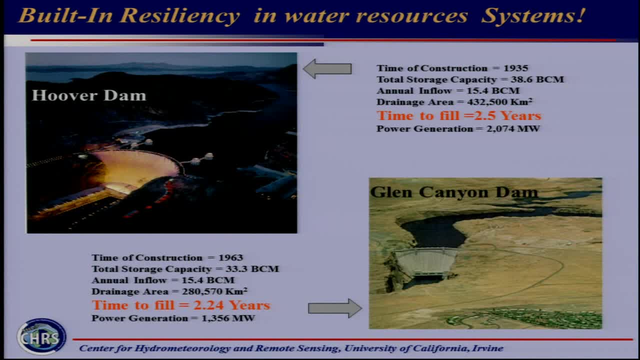 the average time for each of these to fill, based on the average flow of the river, is two and a half years for this, two and a quarter year for this one. So in pictures I showed for 1999, were the good days when both of these reservoirs 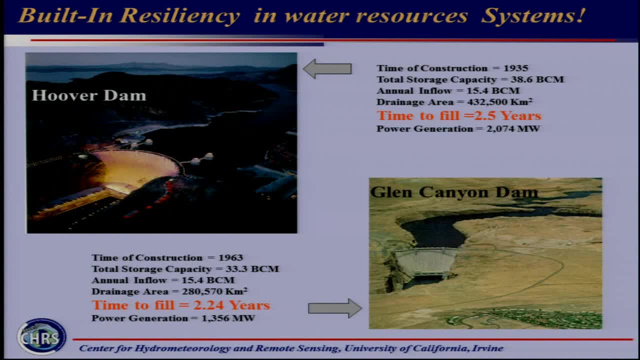 were at the maximum pool capacity, as expected. That means with that much water in the system, you have enough water that, God forbid, you have three or four years of drought. you still will not feel, at least if you live in Los Angeles or Orange County. 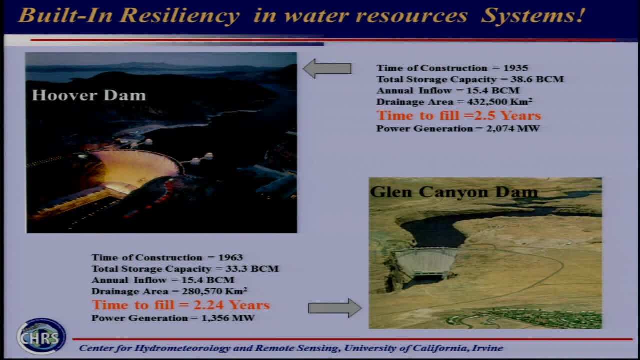 still will get the water because you're getting your appropriation even though the level of the reservoir is dropping, which has been the case in the past three or four years. So we have quite a bit of resiliency built into this. If I compare Colorado River Basin, 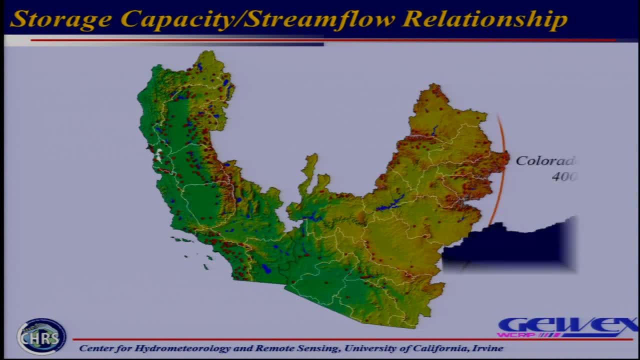 with the northern part of the state of California, where much of our water comes from. in the Colorado River Basin there is almost a 400% ratio between storage capacity and the average flow on the river, So that means you have that much more capacity. 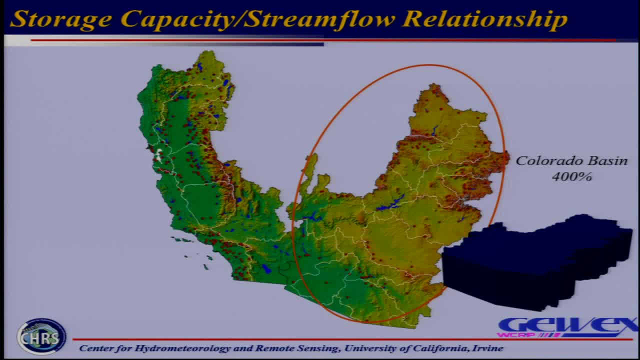 to hold water- okay and for good years that you have a lot of water, so store it. When it comes to the state of California, with the reservoir system we have in the northern part, it's really a one-to-one ratio that you have only enough capacity. 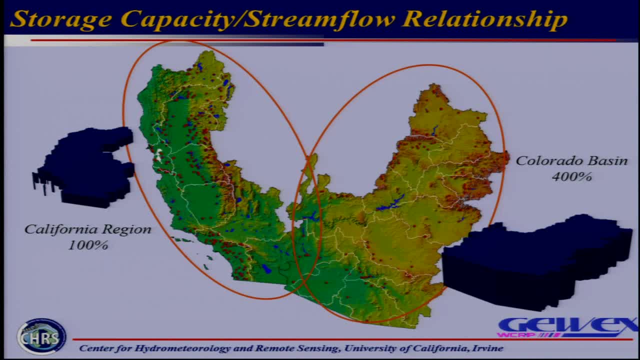 that if you empty all the reservoirs on a good average year of snowpack and precipitation, that at the end of the season you should be able to fill the reservoirs again to the maximum capacity. okay, So with that, the years that we have abundant rainfall. 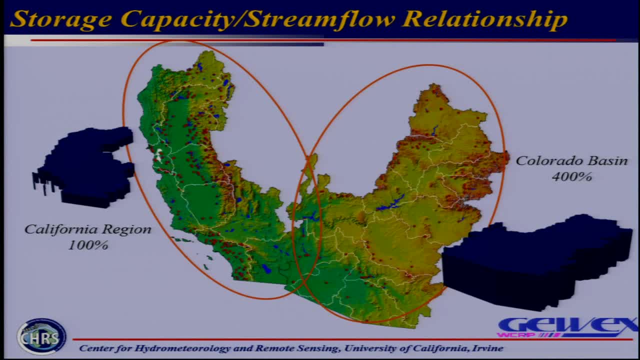 unfortunately we don't have the reservoir to keep it and that's why the floodings happen and for years that we do not have the rain, we don't have much resiliency right After the reservoirs are empty. then we have really severe problems. 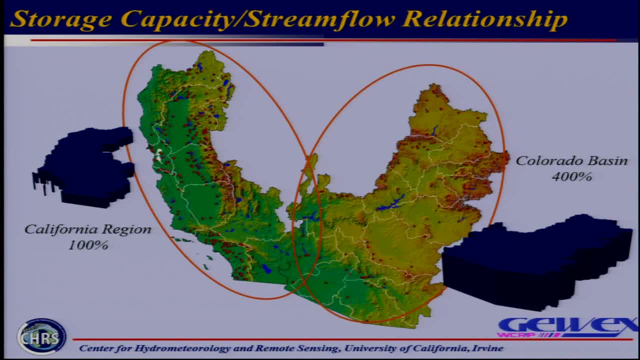 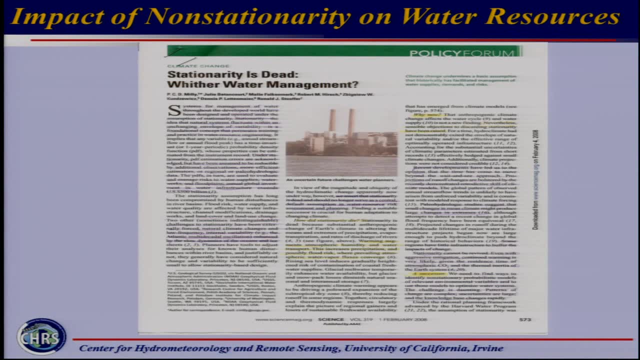 with respect to what to do, and then you resort to groundwater and others. So that's what I mean by resiliency. Let's see what I have: Stationarity. I already mentioned this little write-up in the Policy Forum and Science magazine. 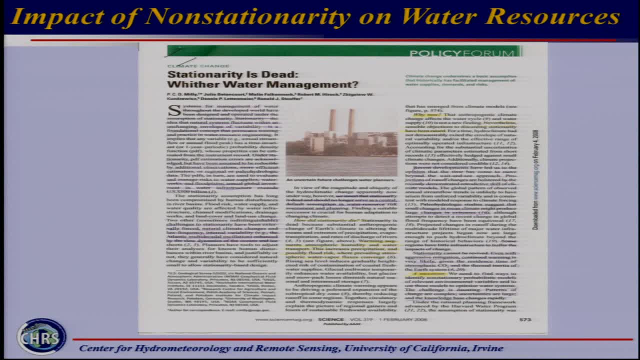 created quite a bit of excitement. that says stationarity is dead with our water management, and I talked to my colleagues. I said: well, nobody argued that stationarity is dead or not. It's the assumption that we make. We know that the system is not stationary. 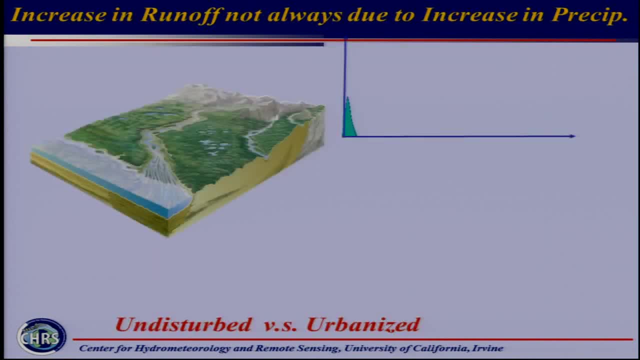 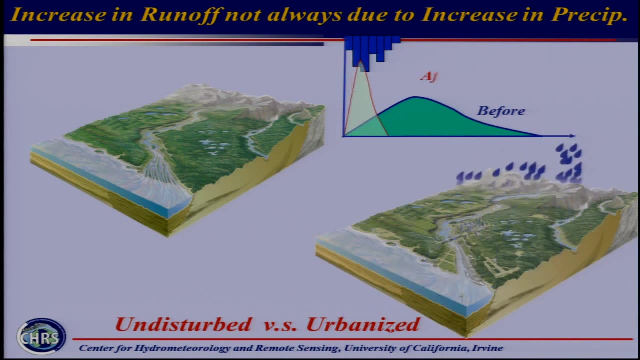 and they agree with that. So why all this matter? is that if I look at- even not the natural climate, as we have developed regions and built more developed regions, building cities etc. the response of a watershed obviously has changed, as I mentioned earlier, 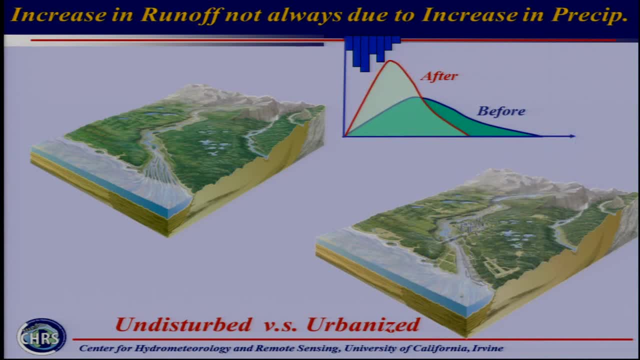 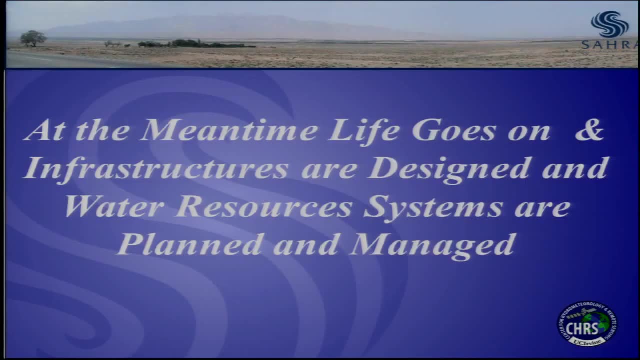 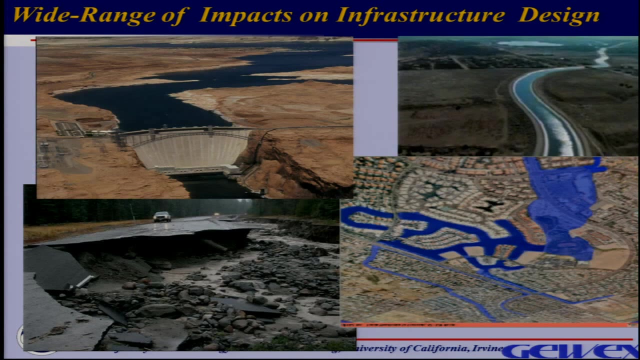 So, whether it's due to climate or not, just the development itself changes the flow patterns and we have not really started addressing these in much of the techniques that we have and we still- life goes on- We've managed as we did before. 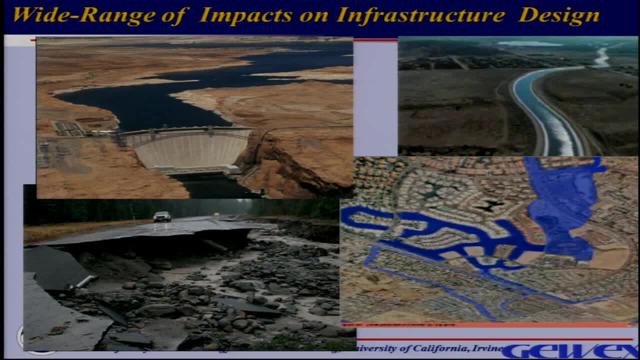 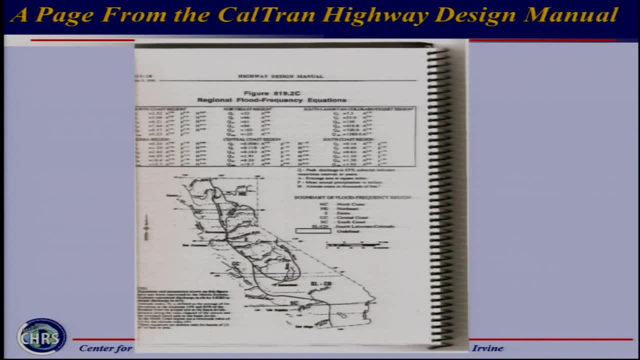 Most of the infrastructure that we have still use the old guidelines, and particularly in terms of the floodplain mapping and urban. If you look at this, this is a page out of the manual for the highway design of the Caltran. okay, So for different regions of the state. 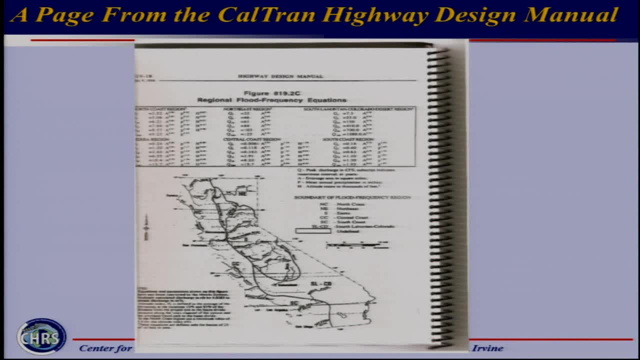 they have different regression equations with their parameters that you can plug in and get an estimate of the 10-year or 20-year flood and then decide your culverts and bridges etc. So it's completely out of date and you know. 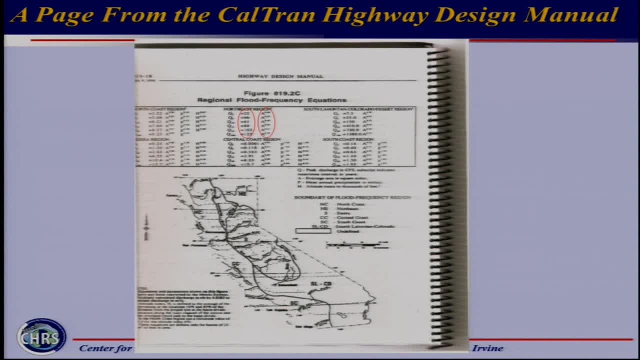 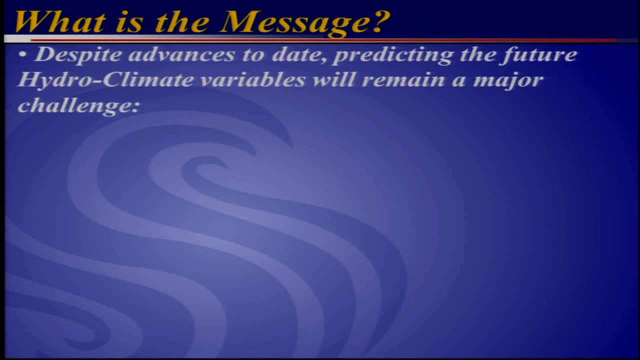 because, as I showed, things have changed And this goes back to the early 70s, when much of this analysis was done and hasn't really been updated. So the good news is at the end of my talk messages: despite advances to date. 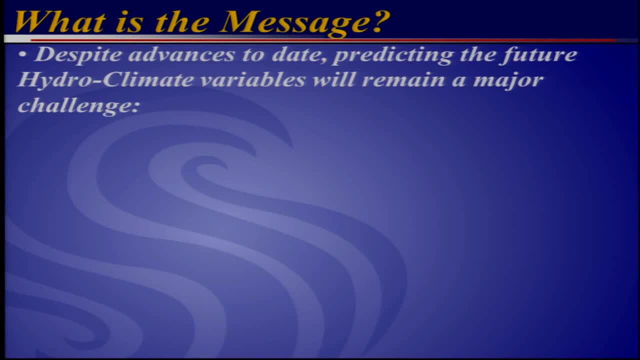 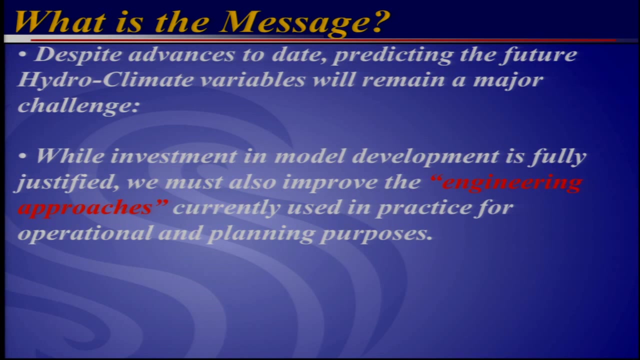 predicting the future hydroclimate variables will remain a major challenge for us, which is, of course, good news because hopefully there will be more interest in the part of the public to also push the politicians and others to provide resources, despite of these issues about whether global warming 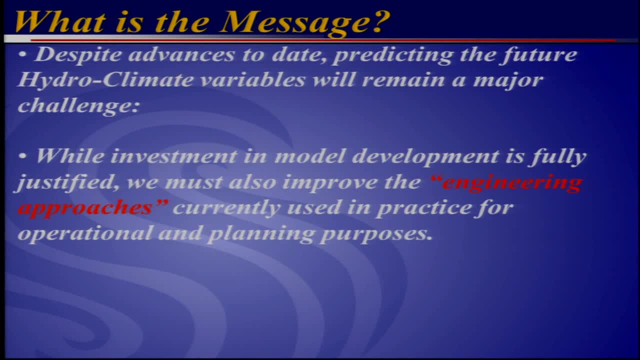 is due to human cause or not, because that's not the issue for us. We have problems. While investment in model development is fully justified, we must also improve the engineering approaches. I think we've let those go down quite a bit and try to. 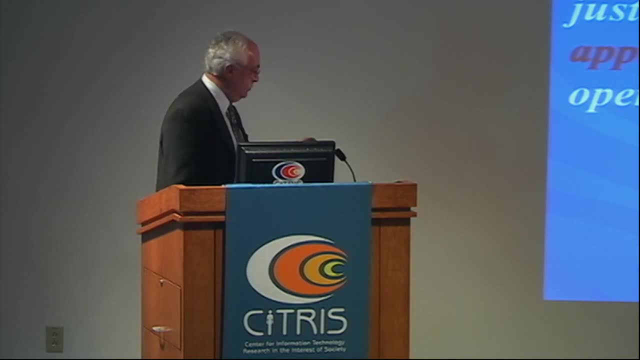 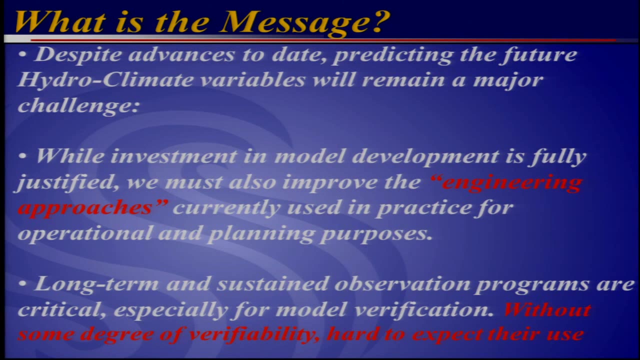 which are used really in practice. A lot of places they still use the old methods. And last but not least is that the long-term and sustained observation programs are critical, especially for model verification and without some degree of verifiability of models, 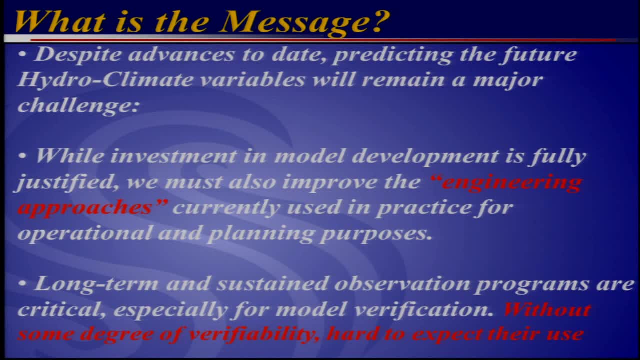 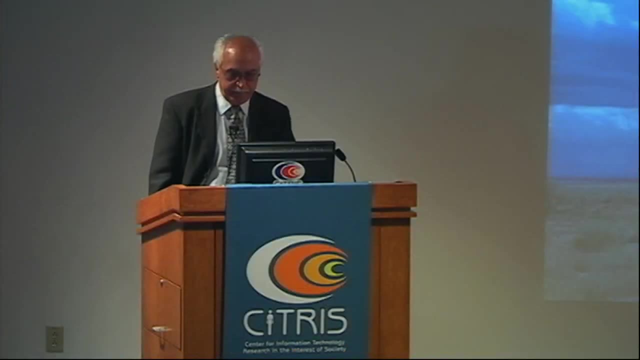 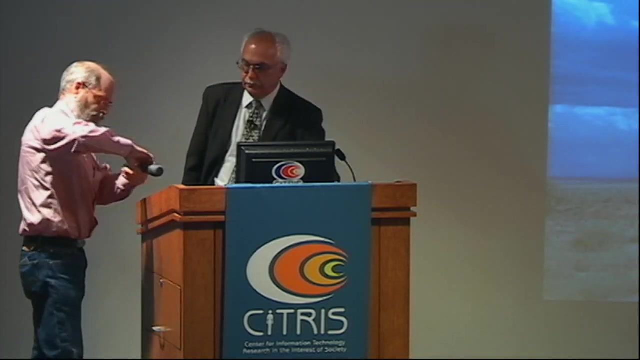 you can't expect people to start using them, and this gets to the heart of what Roger and Steve and others are doing with these various critical zone data studies. Thank you very much for your attention. I'm sorry if I went over time. 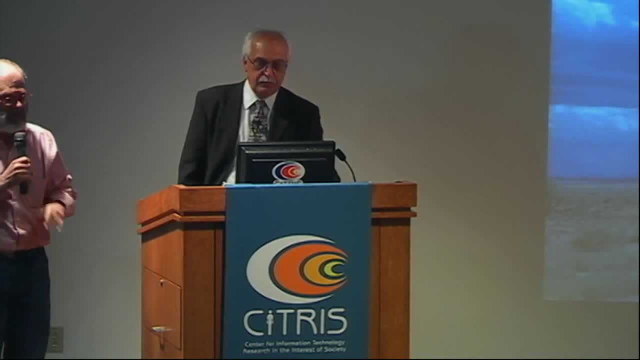 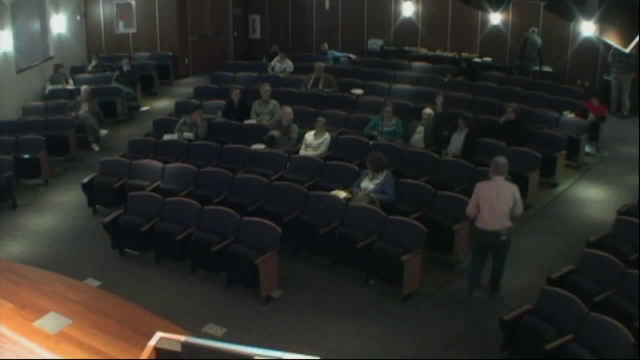 We'd like to thank our speaker. I think we have time for a couple of questions. Well, Saroosh, you did close with a mention of the measurement program data there. I mean, where is the low-hanging fruit, or is there any? 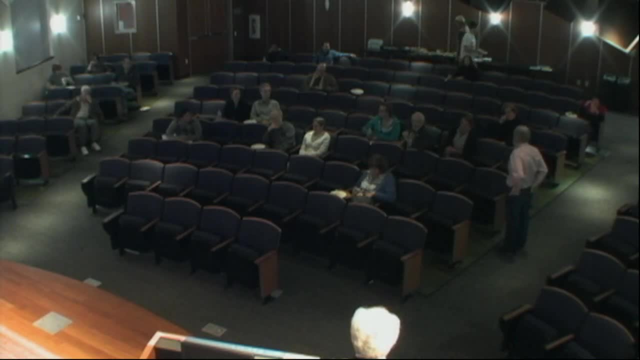 in terms of improving measurements, Because I look at these. you know you contrasted the performance of conceptual versus physically-based models and I know there's been tremendous advances in the modeling, but I really haven't seen the tremendous advances in the spatial data going into these models. 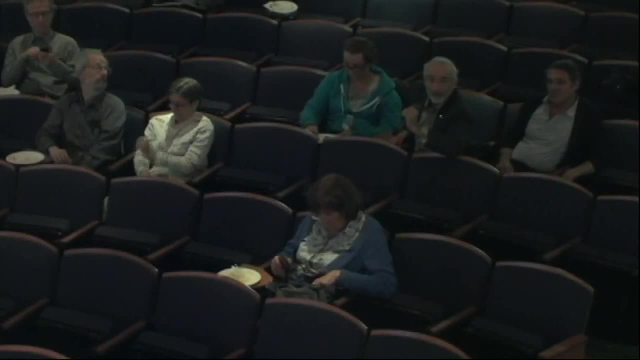 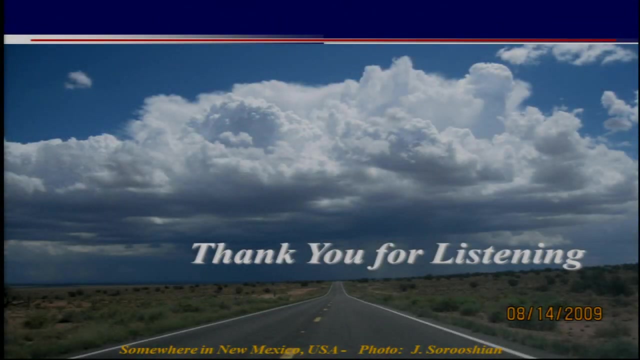 to either calibrate or verify them. Where should we be headed there? Well, Roger, you said it. I mean this has been part of the problem that we think that with a little bit tweaking of the mathematics and giving it more you know, resolution. 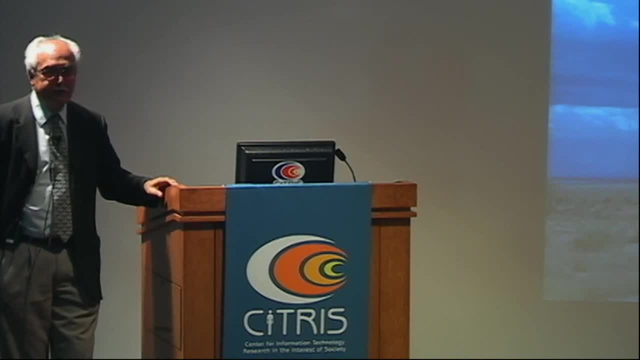 that you solve the problem. but if you don't have the information to feed into those pixels- finer pixels- then you don't really necessarily gain anything. You know you can start from any aspects of it, but obviously from my point of view and bias, 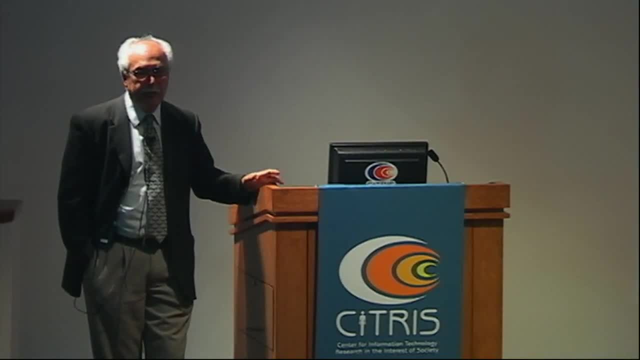 is that precipitation? because that's the primary fuel to the hydrologic cycle. we still suffer quite a bit with respect to the availability of that. Now, you know my group does remote sensing. so do others. I think we've made quite a bit of improvements. But still we don't have the data to verify these things, because if you don't have In Western United States, US has probably one of the best and most condensed rain gauge network of any place and we've got radars. Western US radar doesn't work because we have terrain and blockage doesn't allow you to get the amount of rain. It's in mountainous areas And then the rain gauge density in the Western US is one gauge per 600 kilometers square. 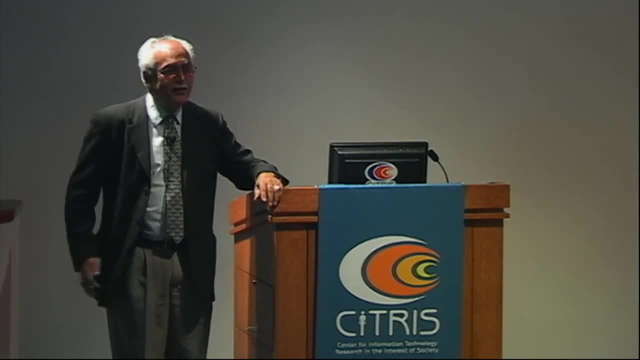 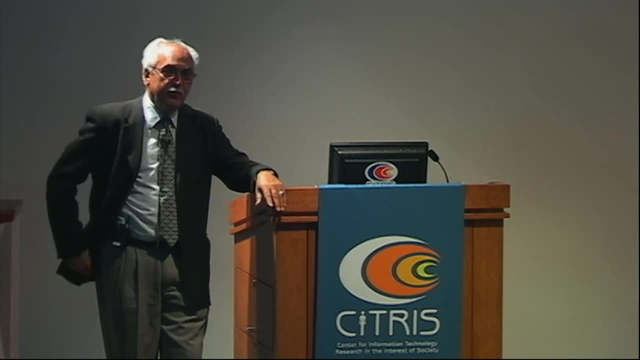 Okay, so think about it. You go 25 by 25 kilometers and you have, on the average, one gauge, and these are mostly near the urban areas, So mountainous areas, where we get most of the rain, we don't get it. 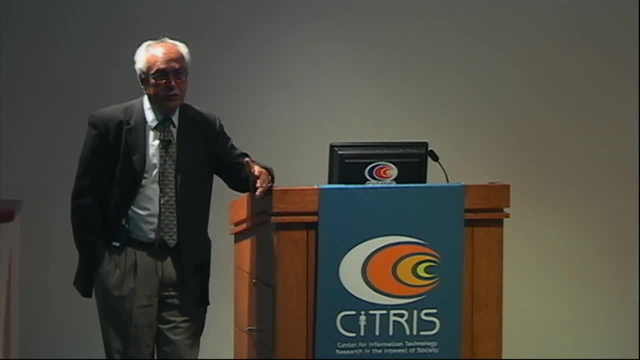 So, Roger, to me that's one area, and then it comes to the heart of how water is partitioned in a model, and this is the type of stuff that you folks are trying to do with sensors to see if we can measure. 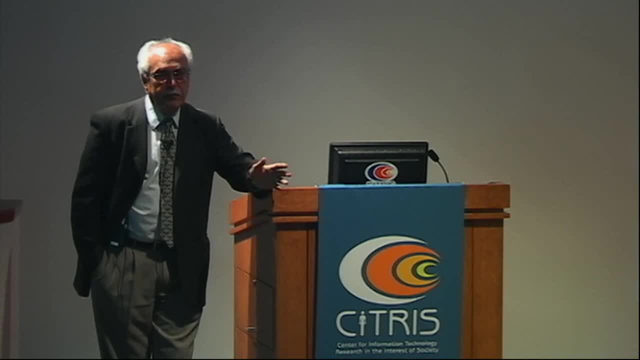 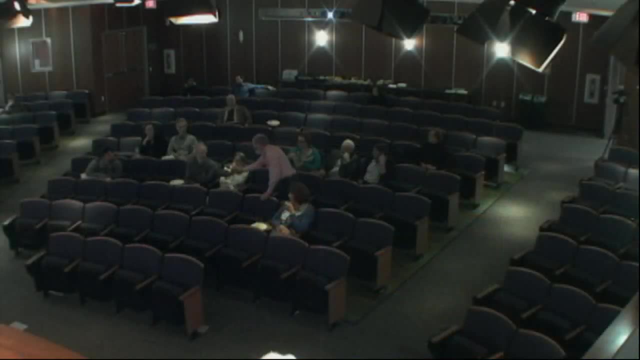 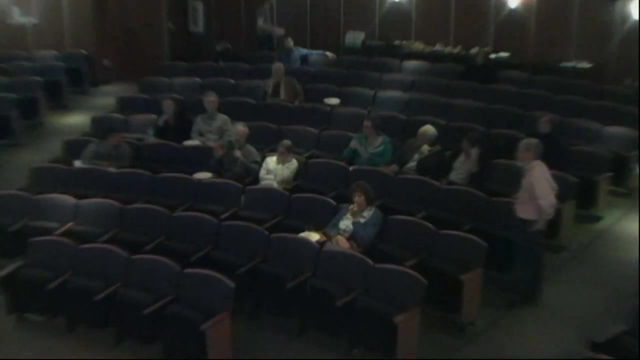 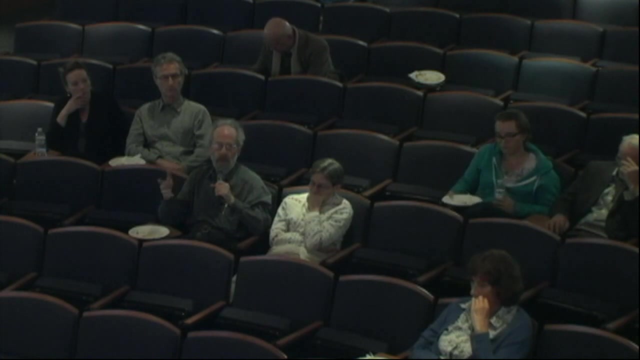 soil moisture better than others. So it's a whole range of things. There are a lot of things that you need to work on. So, in terms of resiliency, do we know anything about the relative costs of building resiliency in the water handling infrastructure? 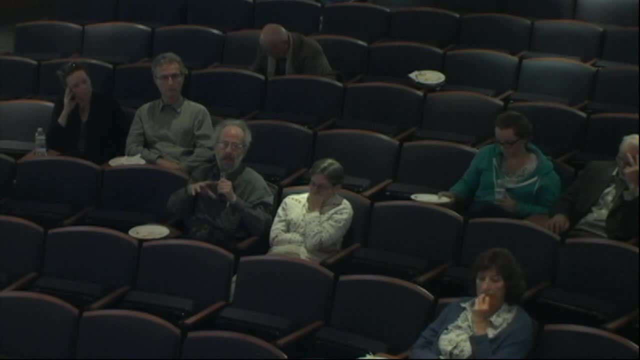 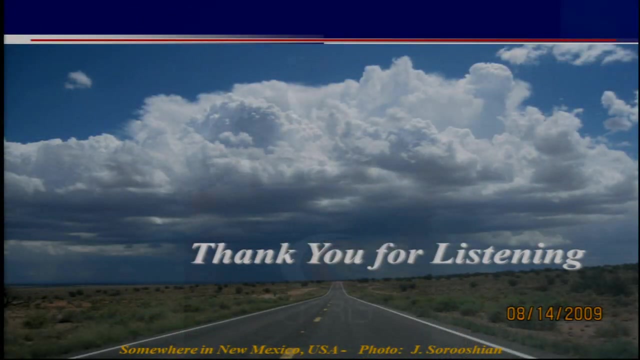 versus building resiliency in the end user built environment, with the buildings, the roads and so forth, as responses to the difficulty of prediction. Yeah, I should broaden the notion of resiliency. It's not always building more capacity and reservoirs. 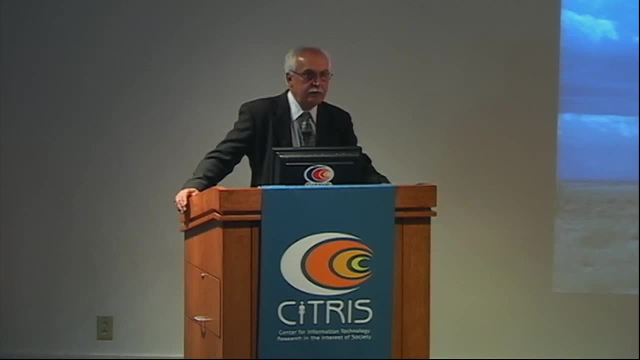 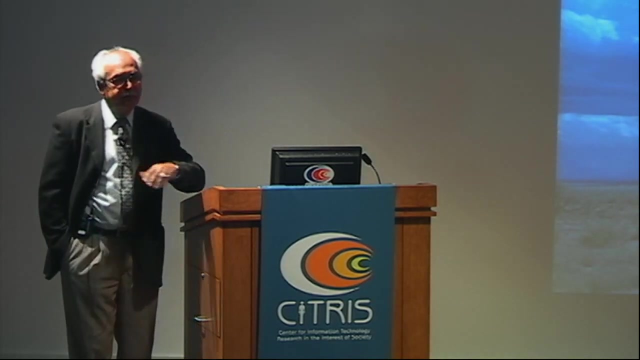 I mean in Orange County, in response to expectations that the state would not give them as much as water they used to get. I mean essentially treated wastewater. almost 90 million gallons a day are being treated to an incredible quality and being sent to the further from. let's say, Irvine area towards Anaheim, and they're being recharged into the groundwater And there are some regulations that you can't use it for a number of years until all the bad stuff is supposedly absorbed by the soil. And now they're increasing that capacity. 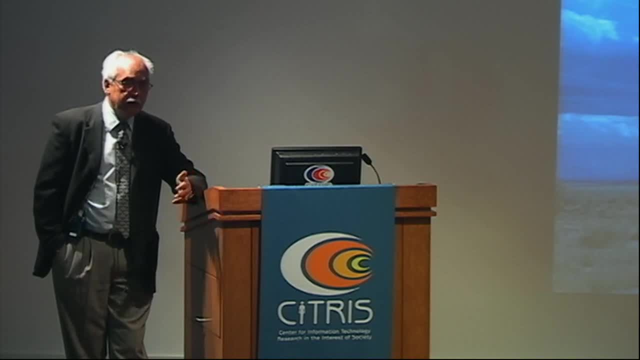 to 200 million gallons a day. So you know, those are to me again adding to the resiliency. okay, Now, in terms of cost estimates, ASCE from time to time tries to do an assessment. 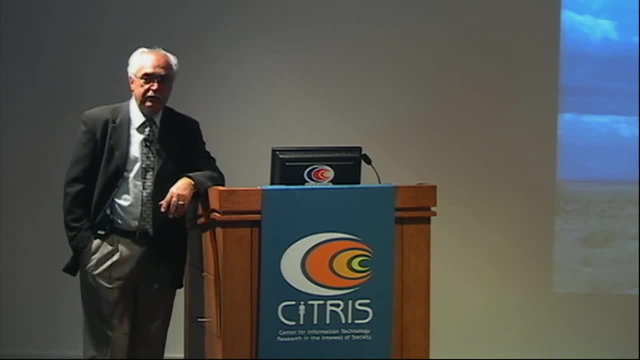 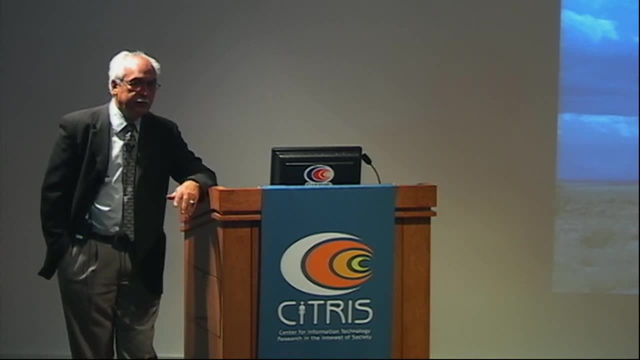 of what it takes even to maintain the existing infrastructure in the system. So I honestly don't think anybody has really given it much thought and doing it, but from my perspective I think it's really important, at least on regional timescales and regional areas. 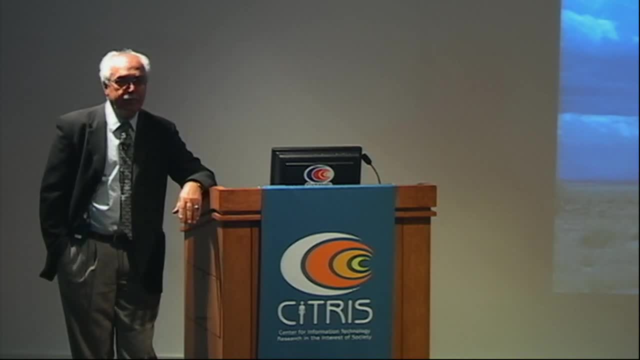 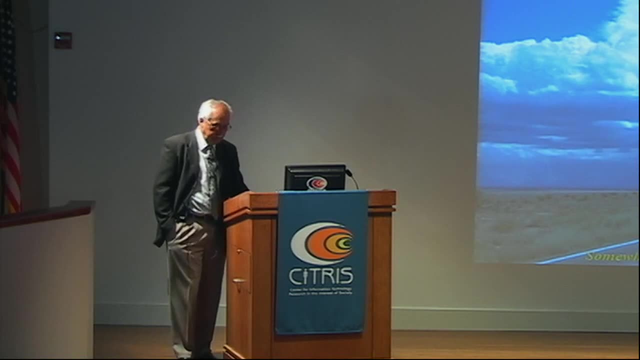 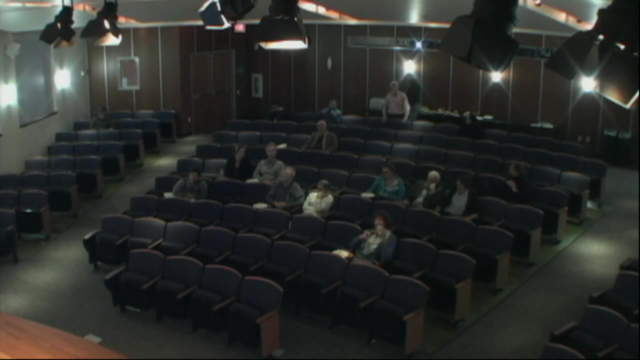 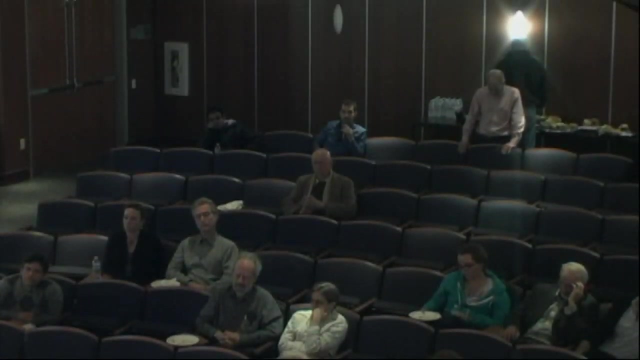 just that this be done. Time for one more. Thanks so much for a really interesting talk. One thing that really caught my attention was the plot you showed from 2011,. the plot that showed that what the users want is not what the predictors can deliver. 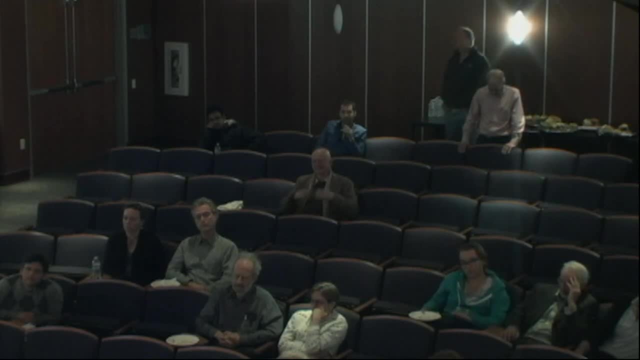 Now this seems to introduce a communication challenge. How Did the meeting where that plot came from? how did you guys conclude was the best way to share this message with people who are often getting the message from other scientists that, yes, I can predict what's going to happen? 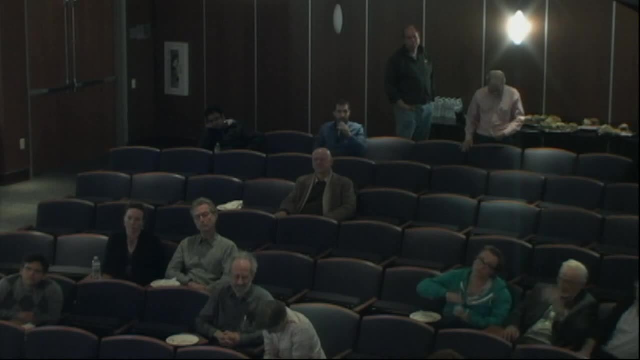 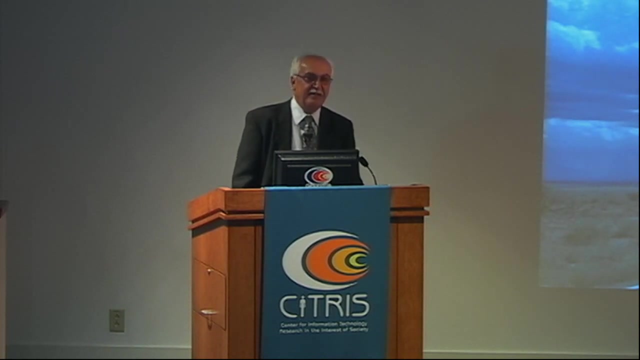 You will have drier summers. You will have wetter winters. If you have a suggestion to make, we're willing to take it Honestly. it's just being realistic and presenting things. It's the right way. Obviously, no restaurant will say: 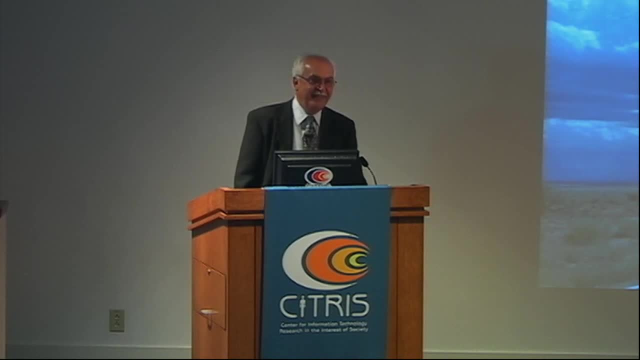 that what they cook is bad, right, But it's the judgment that comes from outside. So I The problem I think we are facing in the community, and I'm not a modeler. maybe Norm is a better person because he's not 100% climate modeler. 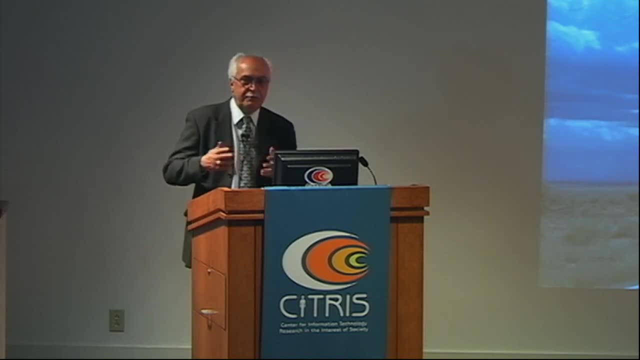 He's a little bit more honest because he deals with people like us hydrologists and others. You know he has to face reality And maybe other among you guys that are in the meeting that feel the same way. I think pushing too much towards saying that. 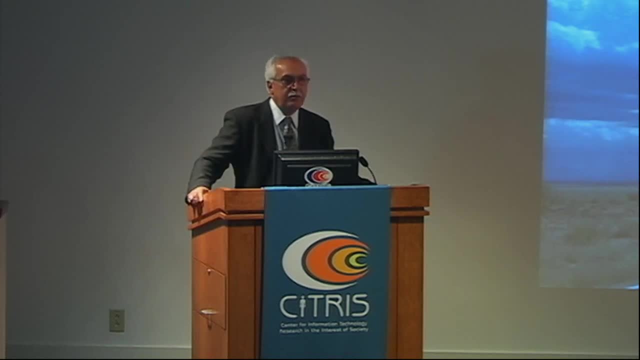 you know, we can predict it's going to backfire on you. Case in point: International Research Institute. IRI was a consortium, at the beginning conceived between Scripps and Columbia University, and eventually they consolidated it all at Lamont. 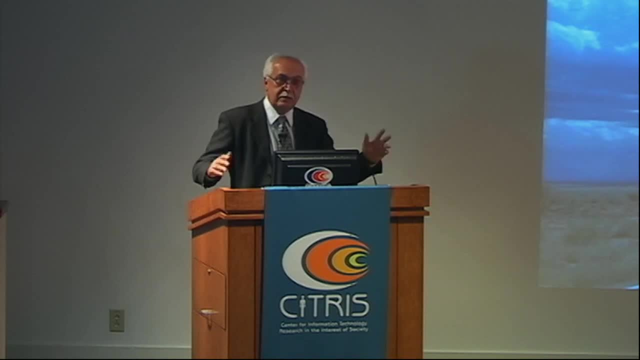 And they are kind of responsible at the seasonal scale And they use a probabilistic and multiple models to predict And they have not really had that much impact to the user community as much as they claim. And eventually this year there was a talk that they were going to be phased out. 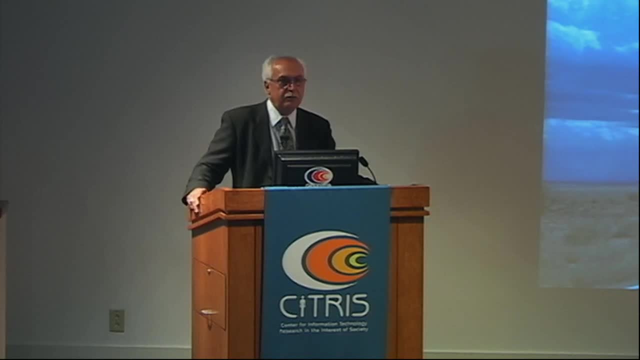 and they lost a big chunk of their funding, Although there was, of course, Columbia University has good lobbyists and they're close to Washington. I think they were able to restore, but they're getting a big cut. So what I'm saying is that going even too far. 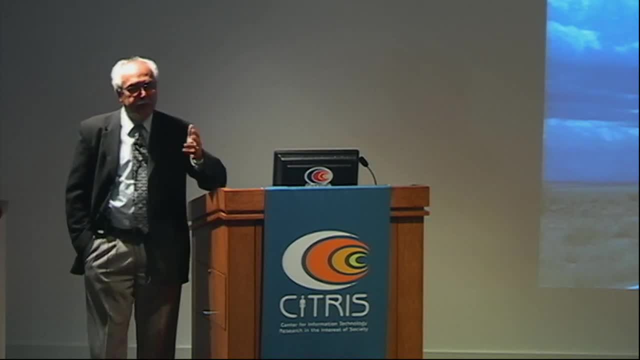 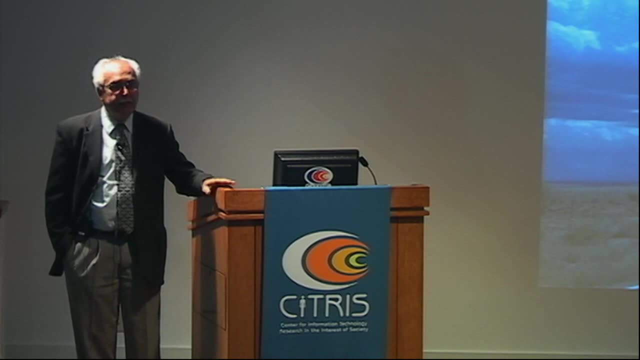 saying that you've got the best product possible eventually will come to haunt you, especially when we're talking about systems like this that are nature-driven right. Yeah, sorry, I wish we knew, But I think there's a lot of people.